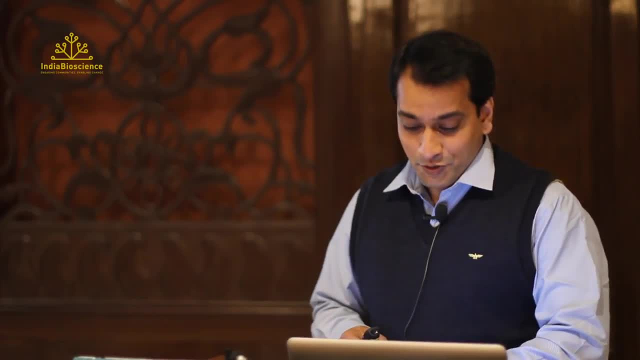 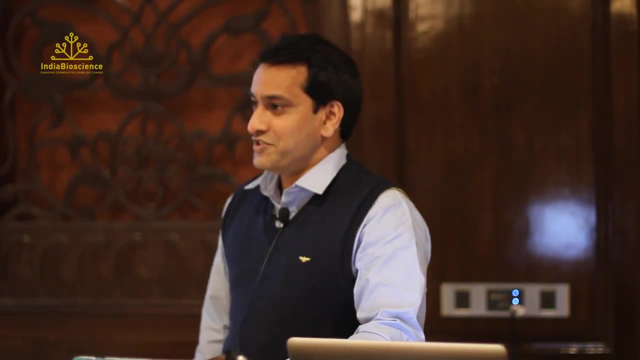 of time, there are more than 10 engineers, So it becomes a package- their own dream as well- And they say no, no, no, no, no. you have to be an engineer and that's where your future lies. 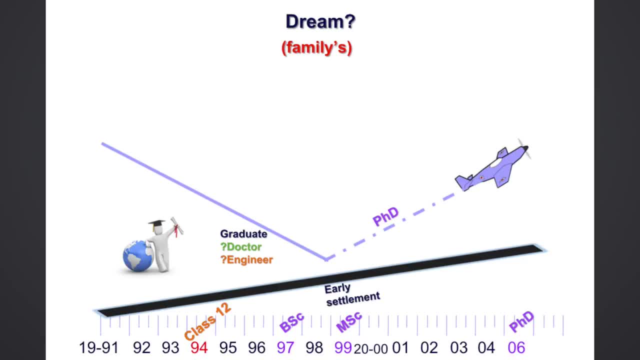 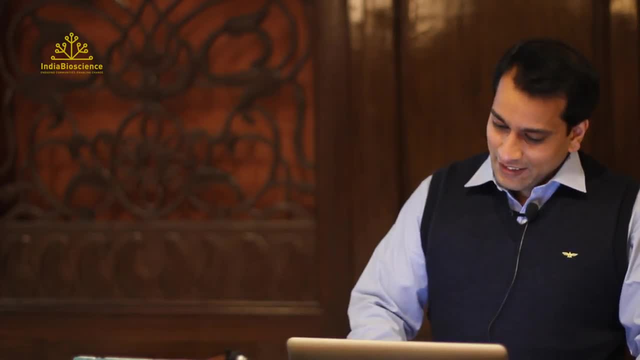 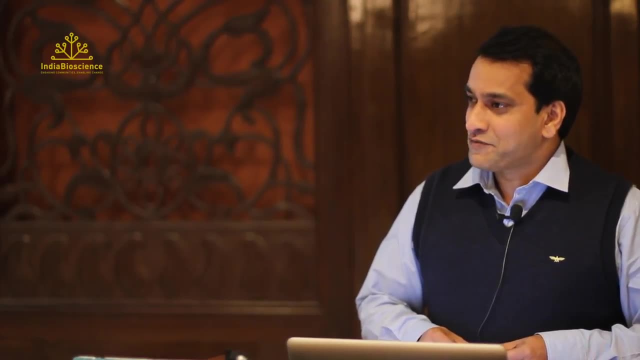 Again, the rebel in me said: no way, I am going to be a physician, so I will prepare for that. This is in my class 10 and 11.. So I did appear for the medical exams from Kutte, Tamil Nadu, Medical Council. The cut-off. 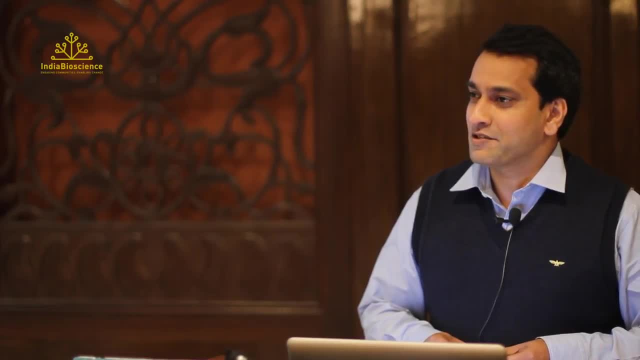 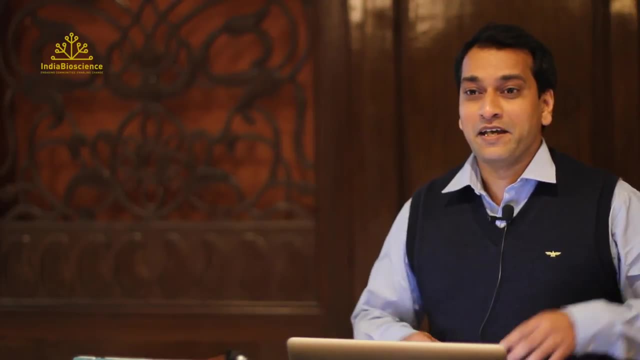 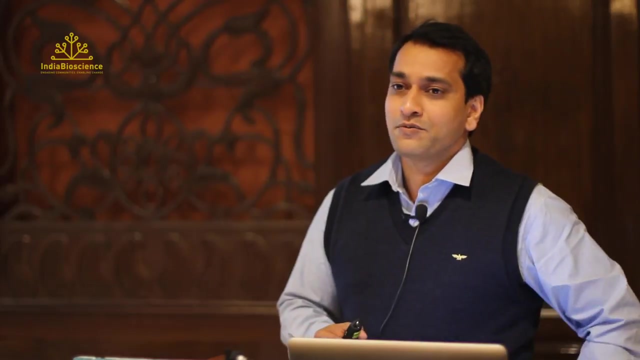 scale. it was pretty much like what we witnessed in India versus Australia semi-final. Close to 300 was the cut-off, and my cut-off was way behind, 85 behind, So I didn't make it So. then the fallback option was to do Masters and Bachelors in. I mean not in that sequence. 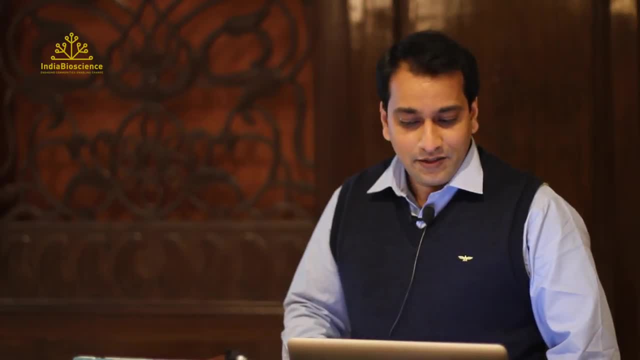 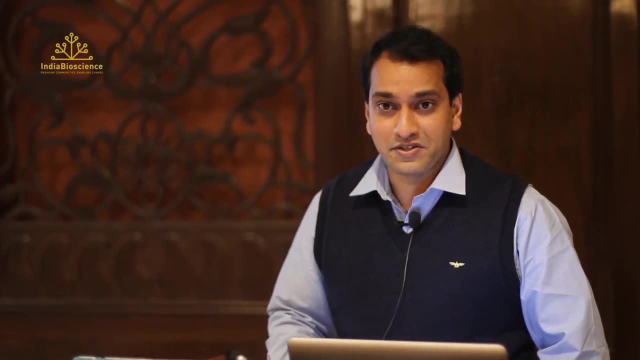 Bachelors and Masters in Microbiology. And then I took off in a completely different tangent, which I did not want to be originally, which was a PhD in Biomedical Sciences And, as you can see here, it goes to the next slide. 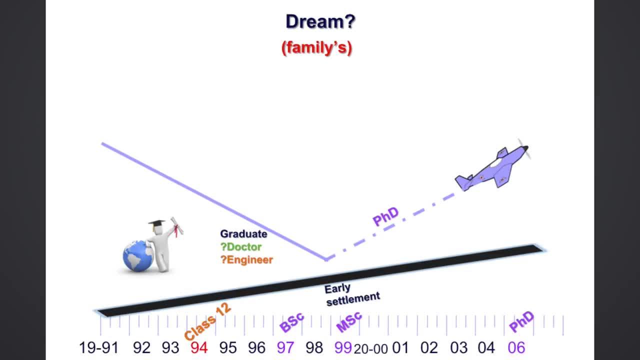 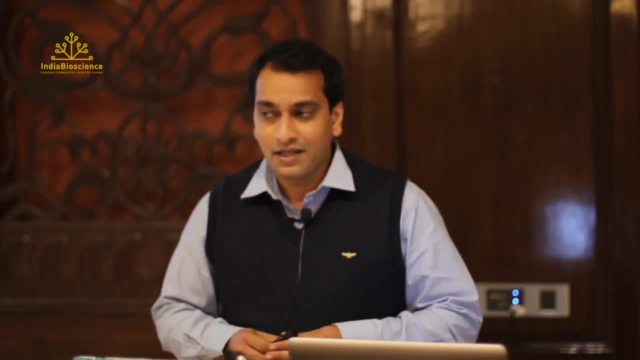 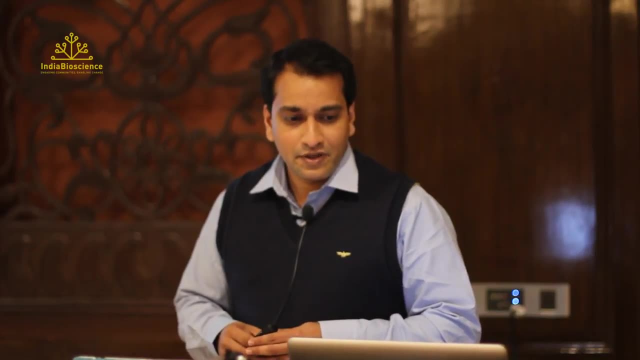 It goes in a completely different tangent as to the early settlement option. So then I joined for my PhD at the Christian Medical College, Vellore, where I worked on genetics of bleeding disorders, And this was for about 5 years, between 2001 and 2006.. I 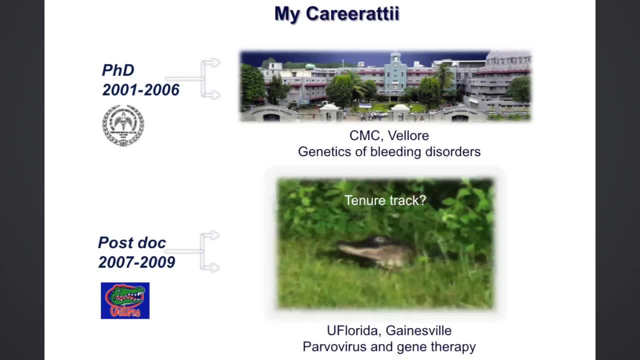 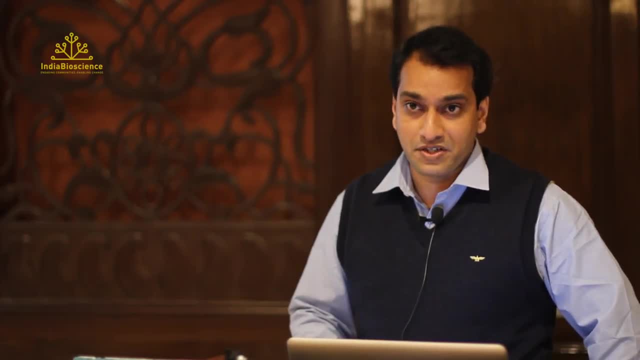 really enjoyed this work. I enjoyed this work because the work that we did has changed the lives of close to about 1000 people, So all of the families who were not families that they could make an informed decision on their childbirth, And these are families with various types of bleeding disorders. 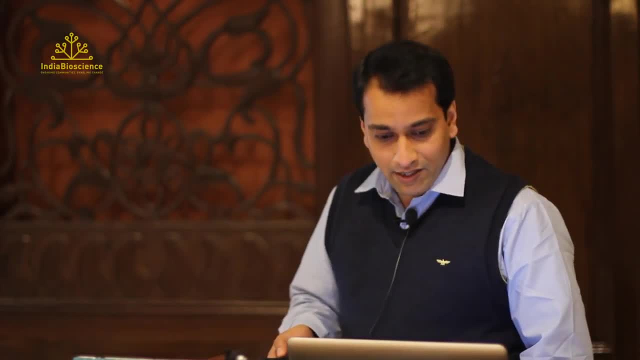 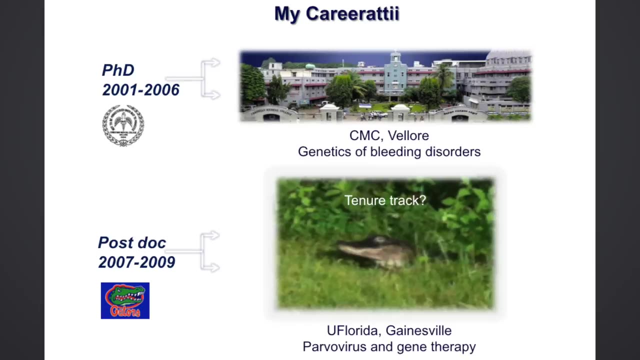 So that was a very satisfying work, And from there I landed up in University of Florida at Gainesville for my work on power wires and gene therapy for a disease condition called Thalassemia. Now University of Florida, MassCade is the Gators. 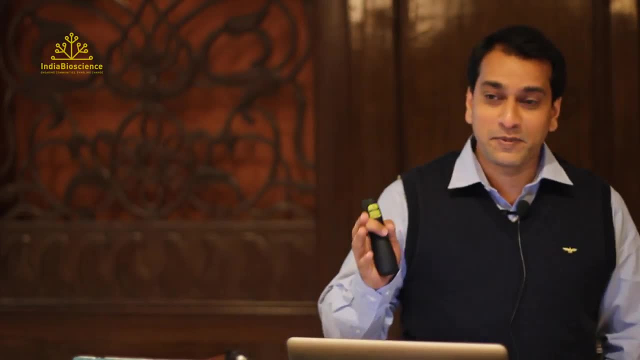 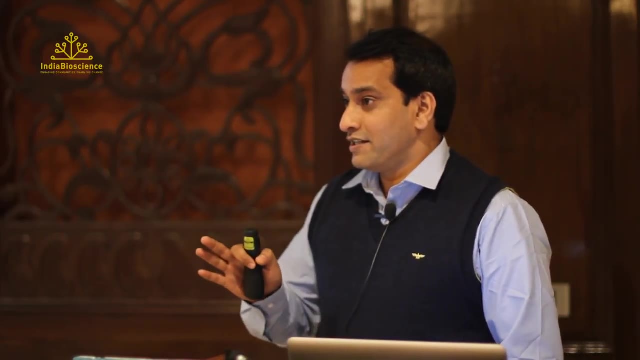 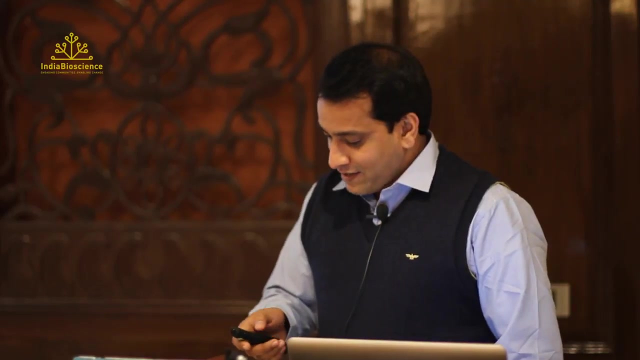 And I proved to be a lucky MassCade for them. This is what my lab mates said, Because the year that I landed up, 2007,, Gators won both the Southeast Conference Basketball as well as the American Football, And some of the Gators also liked me. I don't know if you. 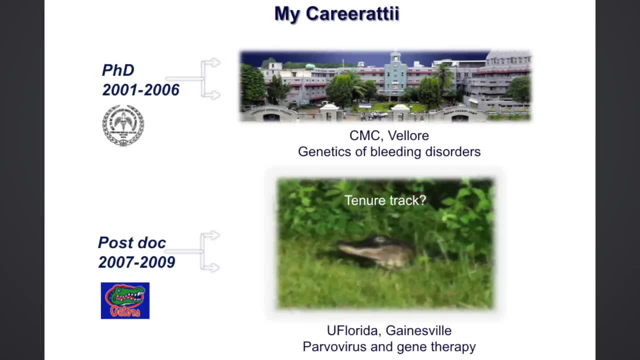 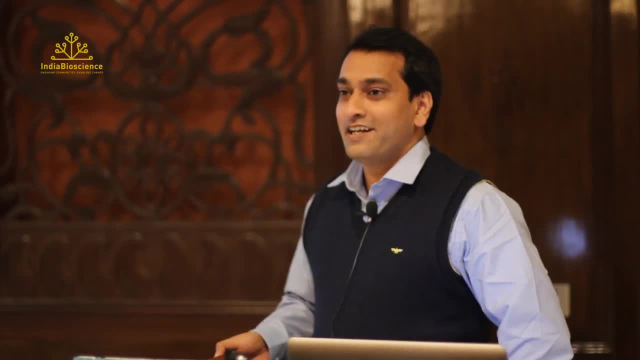 can see a Gator here. They always talked to me when I was walking from my parking lot to the Institute, which is here, And they also offered me a new track. Now I had subscribed to this concept pretty long ago. I said, no way, I have to get back. 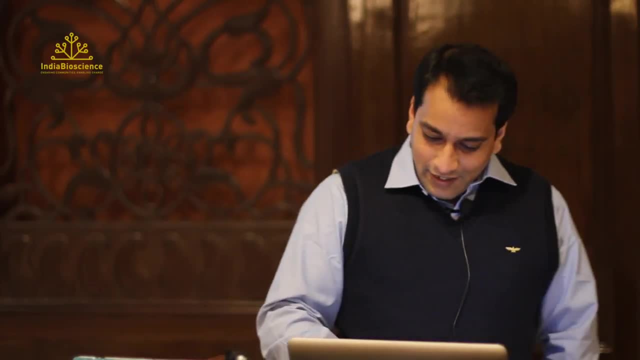 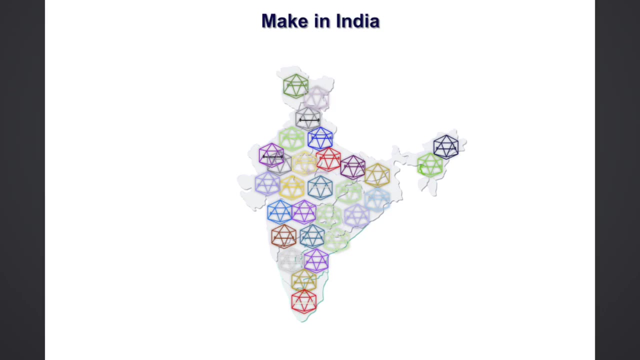 to India and do what I wanted to do. So my first independent position was in Christian Medical College, Belldore for a period of roughly 4 and a half 5 years. 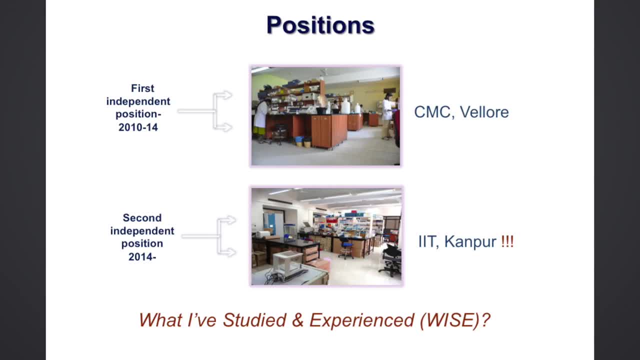 And since the last six months I have been in the Indian Institute of Technology, Kanpur, which, as you know, is a board of engineers, and my family members are having the last laugh here. 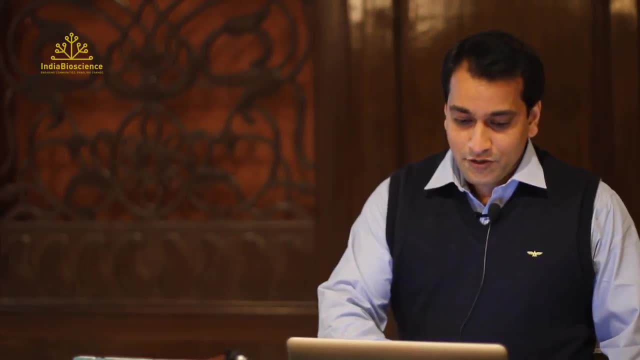 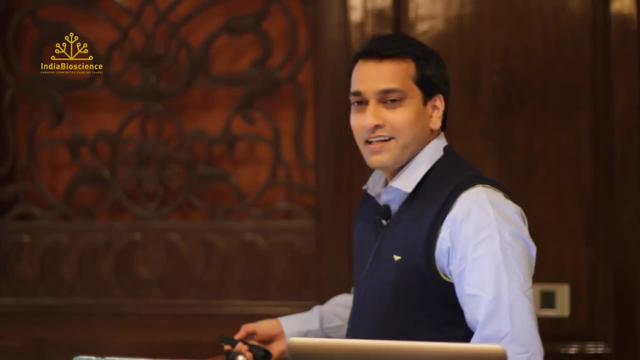 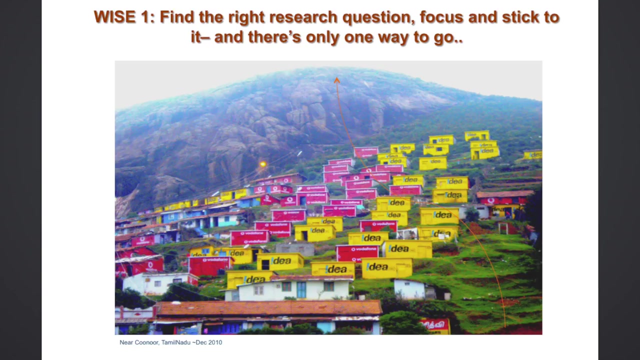 So what I have studied and experienced in this process. The acronym is probably a little bit too much for me, but nonetheless I think what I have realized is to find the right research question at. 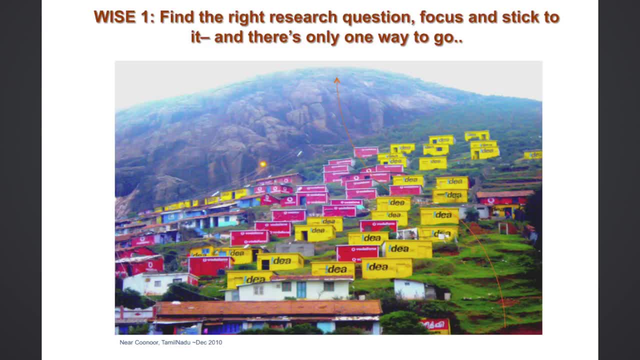 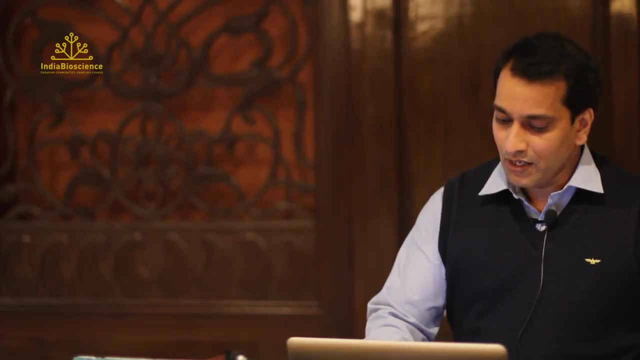 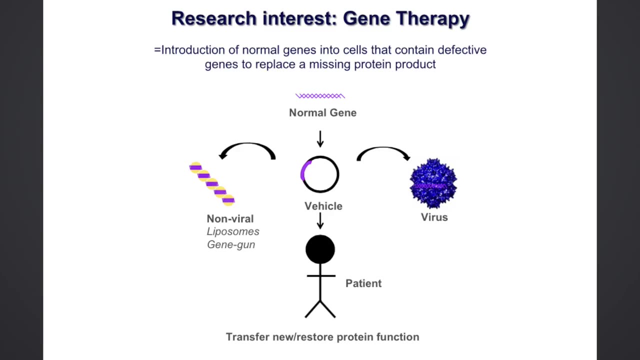 at least when you start with focus and stick to it, and there is only one way to go in your career. So, as far as I am concerned, I stuck on to this topic of gene therapy. For those who are not aware of gene therapy, it is a process by which normal copies of 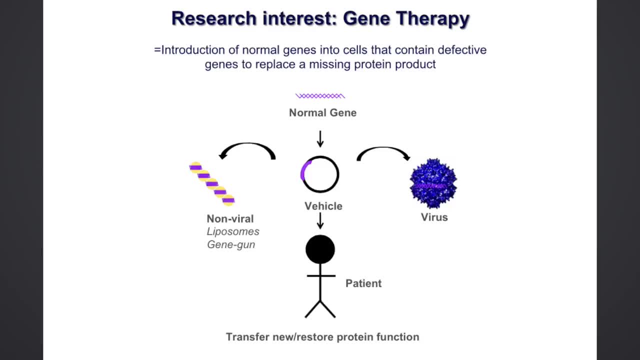 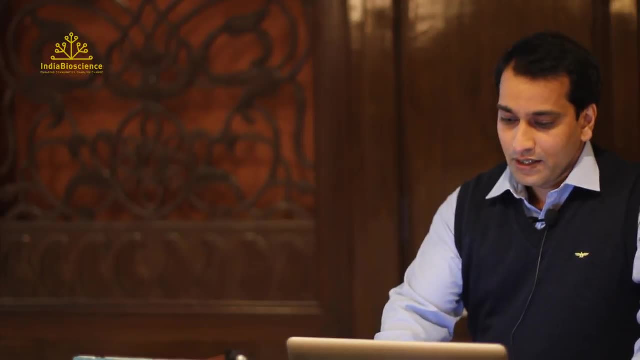 genes are delivered into patients with genetic disorders, So you reconstitute the missing protein function. There are different ways to deliver these genes, but viruses are known to be very efficient because they are naturally evolved to infect human beings. And the virus of my interest was the adeno-associated virus, commonly abbreviated as AAV. 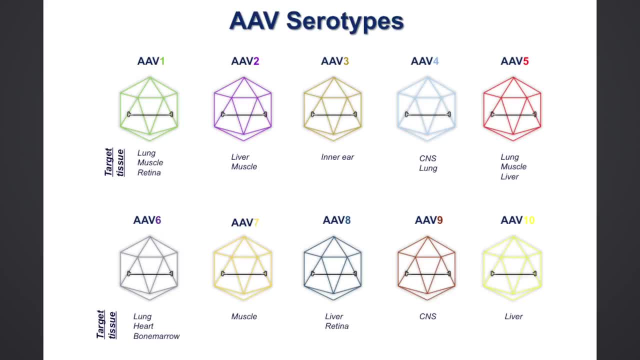 The vector is very minimalistic. The virus contains two genes that are red- that in course, for the replication-dependent functions of the virus, and the cap- that in course, for this capsid protein. It is one of the smallest viruses known: measures just about 20 nanometer in diameter. 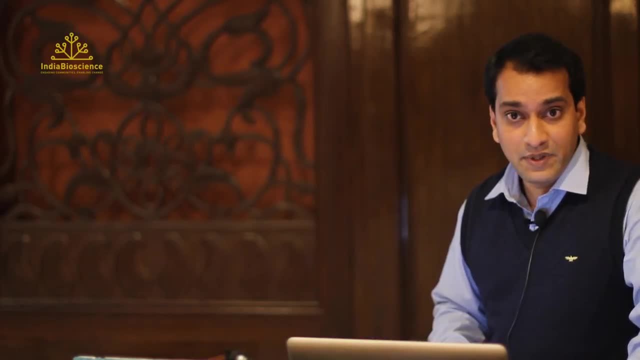 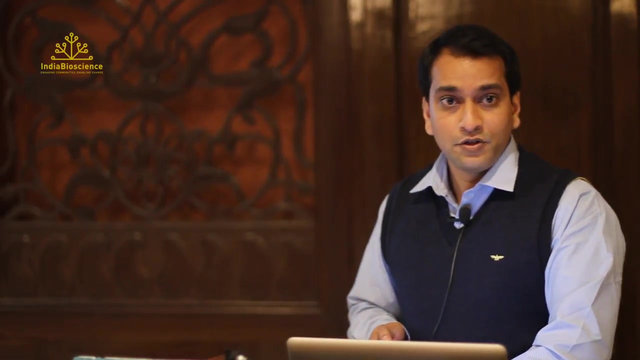 The biggest advantage in the gene therapy field with parvovirus like AAV is its non-pathogenic nature. You and me are positive for this virus, but we don't suffer from any disease, So you can cut the wild type genes and replace it with your cargo of interest. to make this. 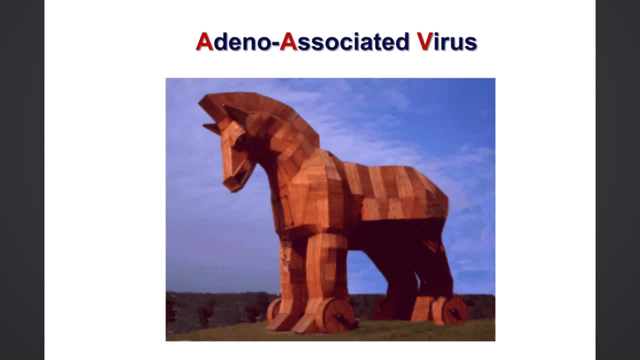 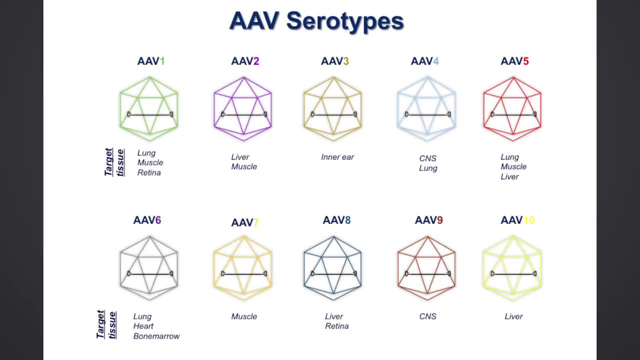 as a recombinant gene therapy vector And basically this is your Trojan horse. And 10 such Trojan horses are known called AAV serotypes 1 through 10. And each of these viruses have their unique capsid sequence and structure that gives them 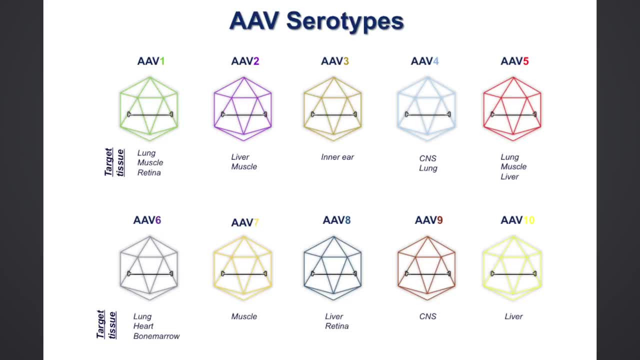 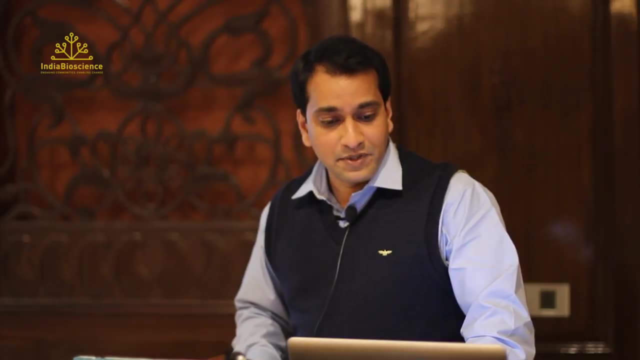 the ability to target multiple tissues in the human body. For example, my interest is in liver disorders And I always tend to use AAV2 and AAV8 serotypes, which can specifically target hepatocyte receptors. Now these properties have been used in various preclinical and clinical studies. 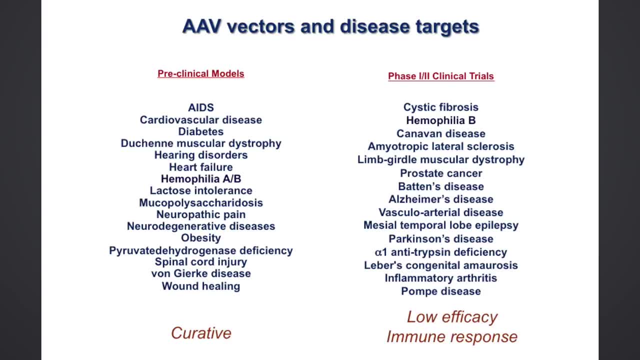 The bottom line is this: in preclinical models, in urine models, everything works fantastically well. When it comes to humans, we now realize that the efficiency could be much better, And there is also an immune response that is directed against the viral proteins which 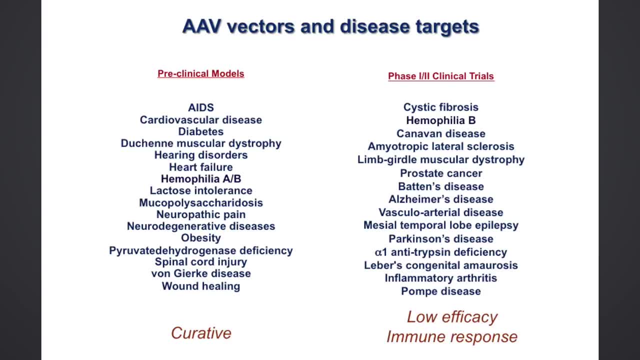 was not seen previously in preclinical models, just suggesting that mice are not humans at all. So, as a case in example, where I work on is in hemophilia, And most of you know hemophilia is a bleeding disorder. You could have spontaneous bleeding episodes which could be life-threatening. There are recombinant factor supports which are available but might cost upwards of $100,000 per year if you want to give a prophylactic regimen, And that is beyond the reach of many. So gene therapy is an attractive option because it gives you long-term cure. 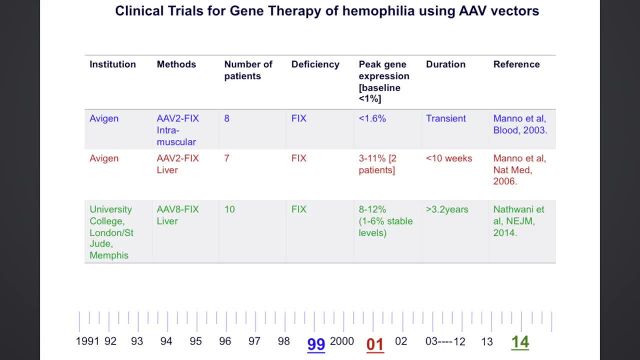 Three clinical trials have been done for a hemophilia B, and they have used two liver-specific vectors, AAV2 and AAV8.. But if I want to summarize these studies, these studies have established the safety of these vectors for gene transfer. 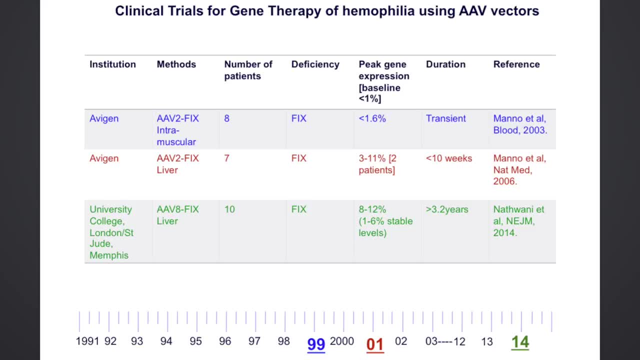 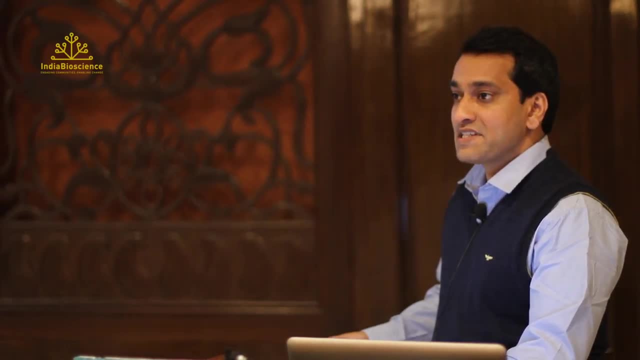 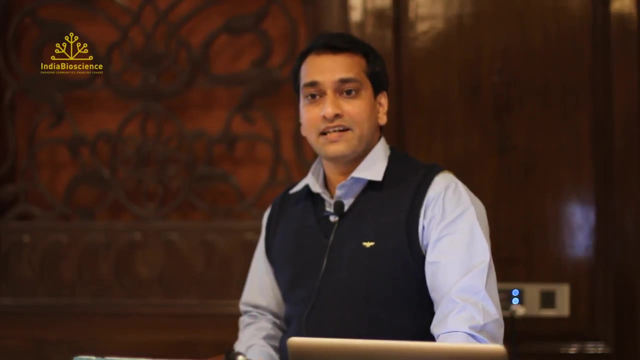 But in terms of what they could achieve, they have achieved only modest efficiency. If 100% is normal, what you get with the currently best available gene transfer is only about 10%. And there is also another problem: There is a myriad of cellular responses directed against the virus. 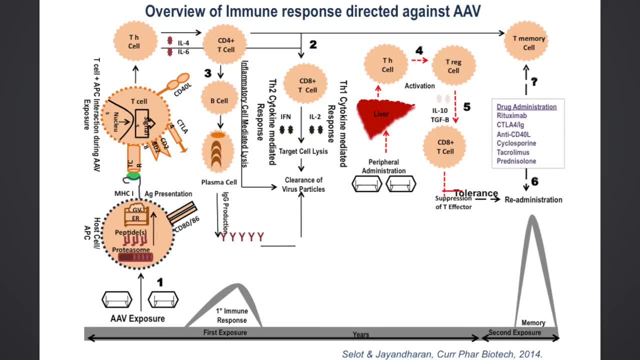 I don't want to get into the details of all of this, but essentially it could be a CDAE-mediated T-cell response that wipes out the transduced hepatocytes. It could be a memory B-cell response. This is due to immunoglobulin class switching, which makes re-administration of the vectors. 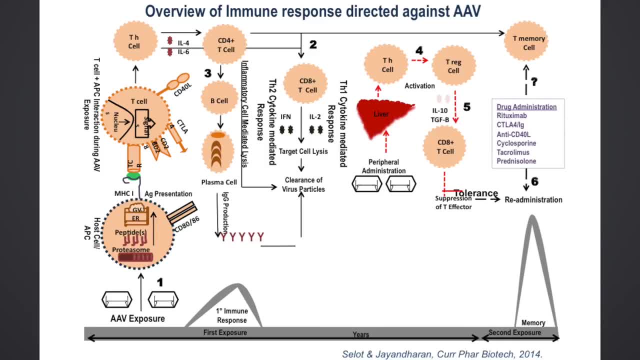 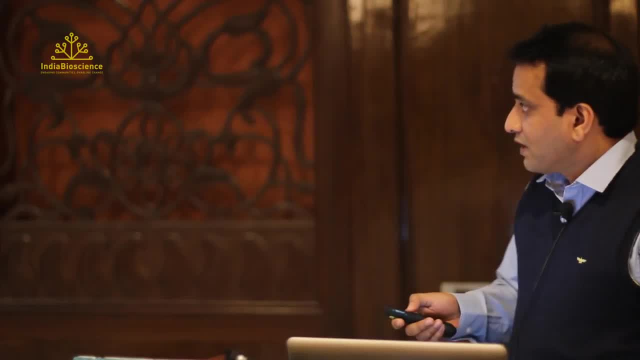 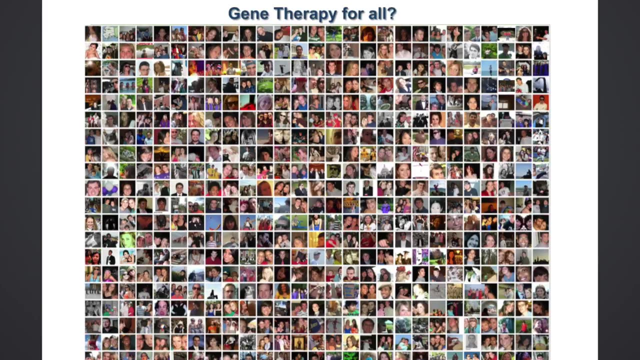 very difficult. In addition, I told you that the majority of humans are 0 positive for AAV vectors, and close to 60% of humans are So, which means that all humans may not be candidates for this mode of gene transfer. It's a very promising system, but the moment it excludes a majority, it ceases to be something. 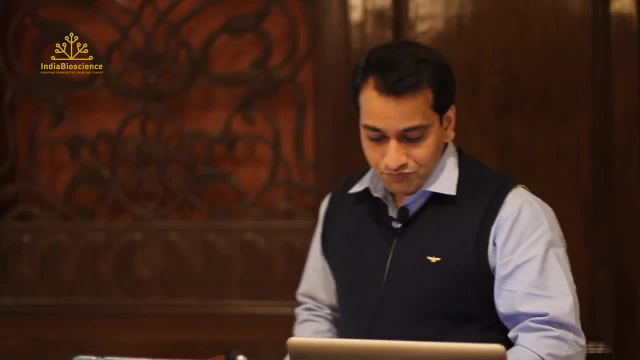 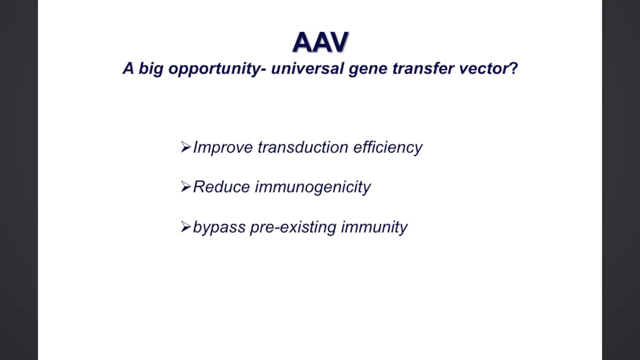 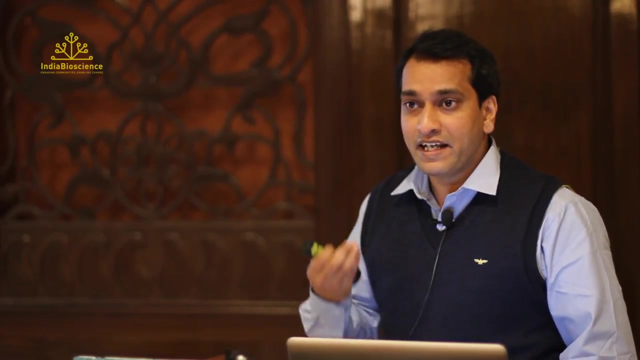 very useful to become a standard of care. So we had a big opportunity here at multiple levels to make this vector system a universal gene transfer vector, so that one could improve the transfection efficiency, reduce the immunogenicity of these viral vector systems and also bypass pre-existing immunity by developing what is 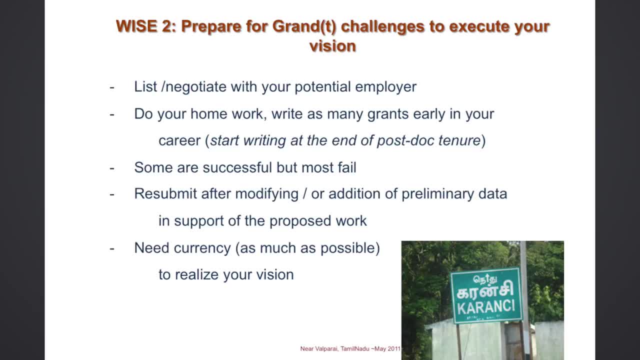 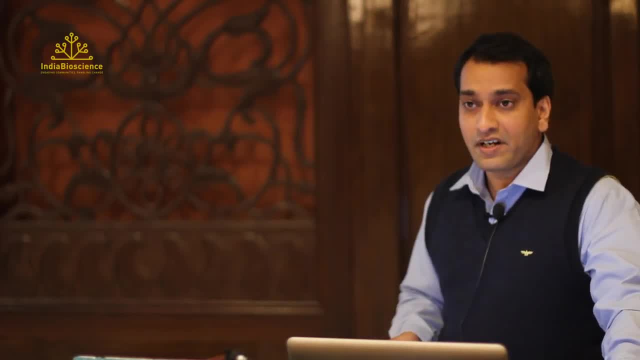 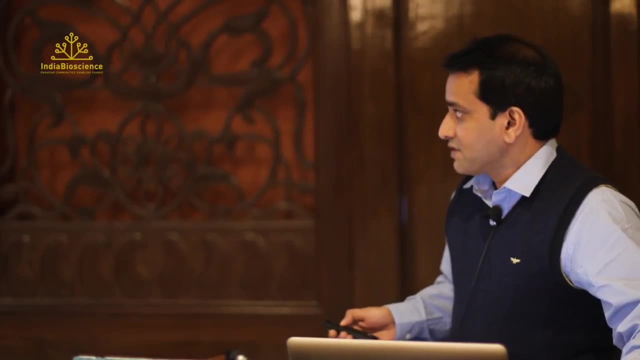 called as immune-stealth vectors, And my lab focuses on these parameters. The research focus of the lab for the last six, five and a half years has been trying to understand the biology of the virus and the host-cellular interactions at multiple levels. 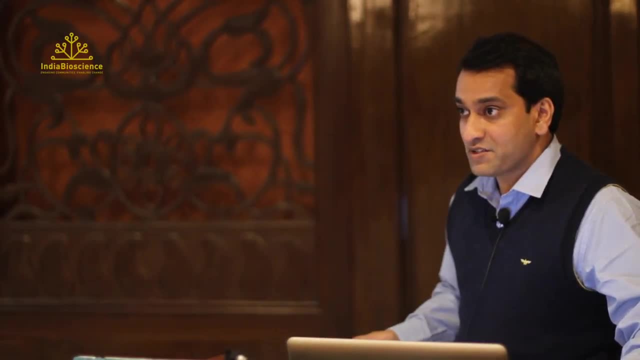 The various cytoplasmic surveillance mechanisms and nuclear surveillance mechanisms, so that we understand the processes which are detrimental to the gene transfer with AAV vectors. Now, with this information, we tinker specific aspects of the virus and the host-cellular life cycle. 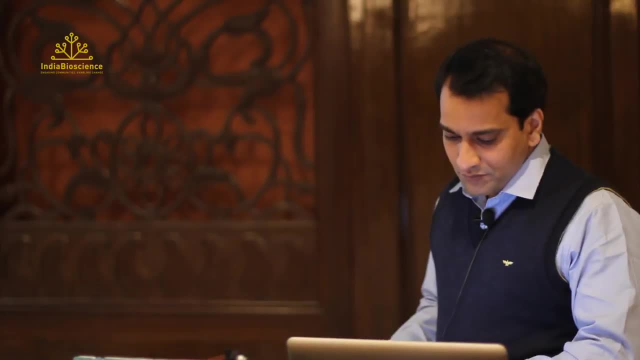 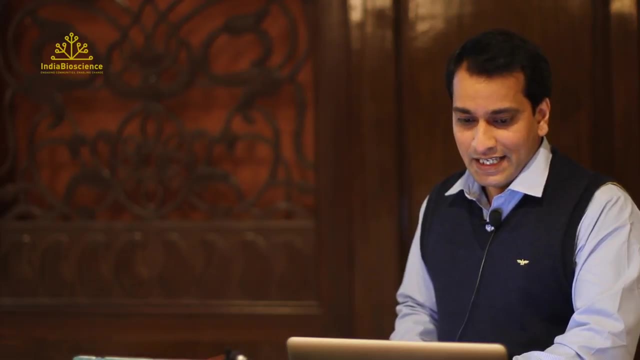 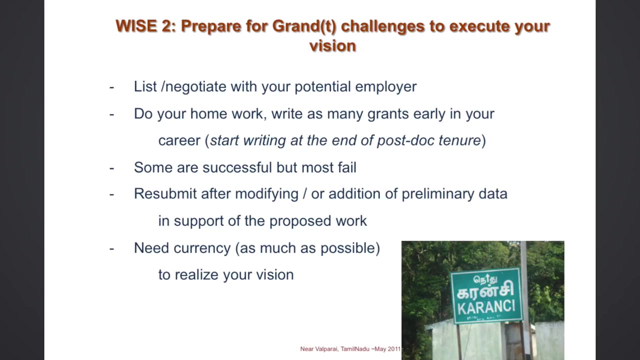 To make better gene therapy vectors, And, of course, we use a variety of model systems that are listed out here. So you can have grandiose vision, but at the end of the day, you need money to execute them, And one of the things that I learned pretty early is prepare for your grand challenges. 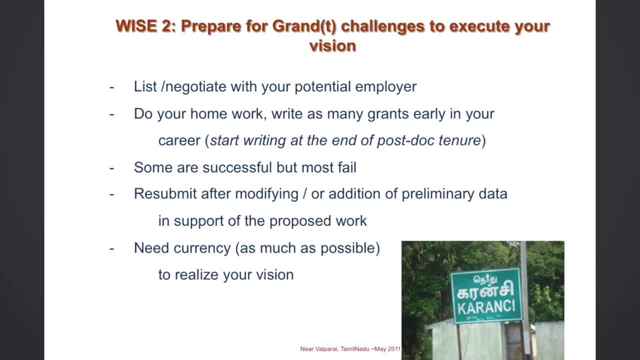 as early as possible. Of course, if you are young postdocs who are trying to migrate to your position back in India, list what you need. negotiate with your potential employer, do your homework, write as many grants as possible early in your career or when you are just finishing. 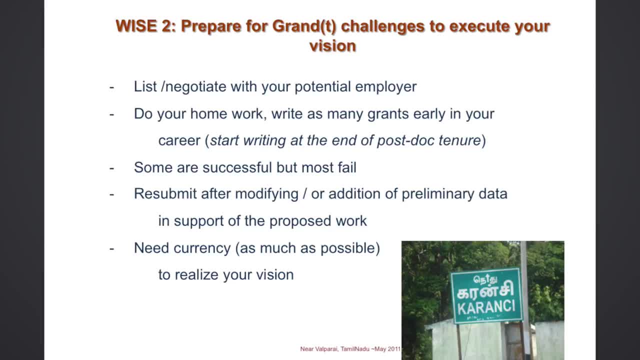 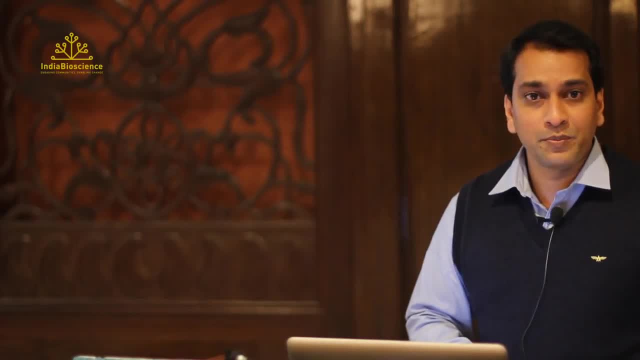 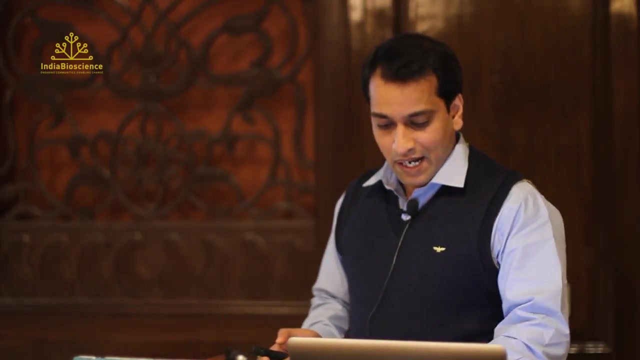 off your postdoc. You save a lot of time there. Most fail- You have heard this from previous mentors as well. But it also gives you the opportunity to understand what went wrong. try to modify them and resubmit them And at the end of it you need currency as much as possible to realize your vision. 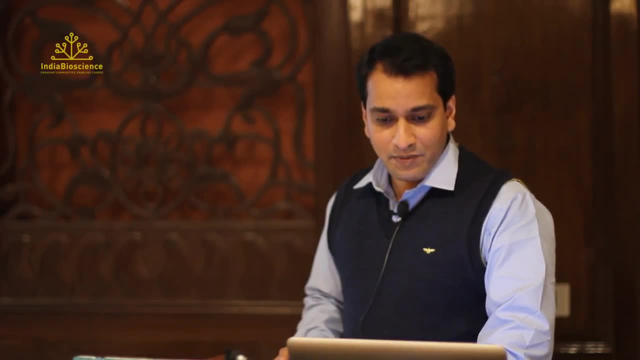 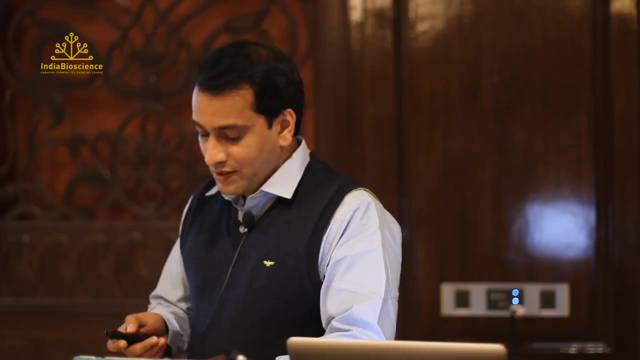 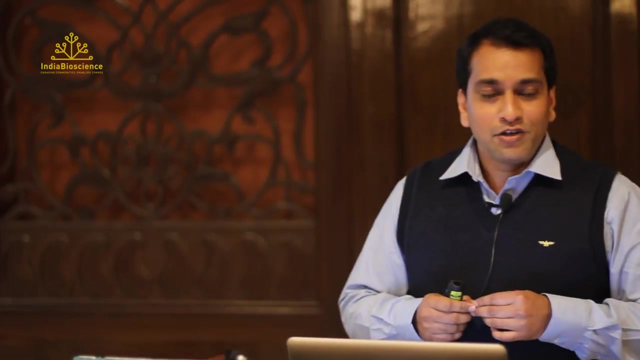 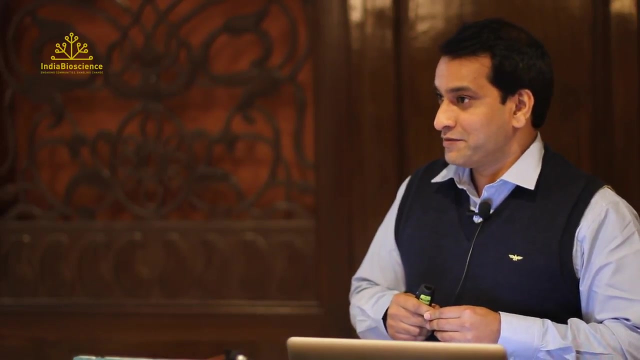 So I was fortunate because I did submit one of the grants just before I moved back to India. This is a couple of months before I landed in India, And within six months we could get a $200,000 grant from Bayer. It also helped me self-motivate because I now believe firmly that I belong there from. 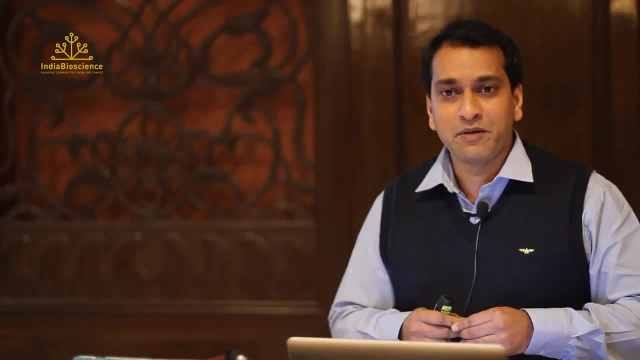 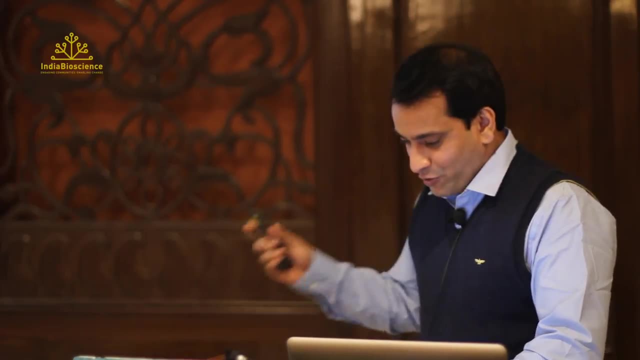 a postdoc to a PI in getting an independent grant. So this has shaped my vision from there on And of course since then it has been quite a lot of grants written up, Some of them supported, Some of them compromised. 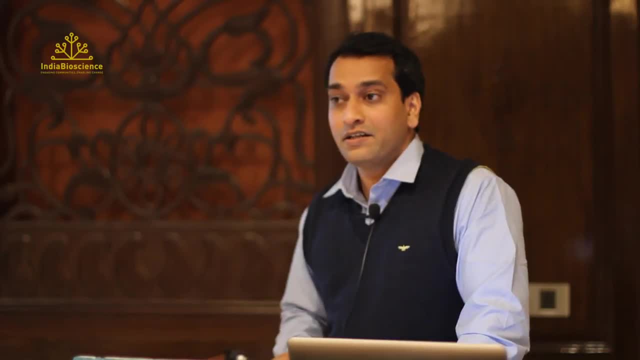 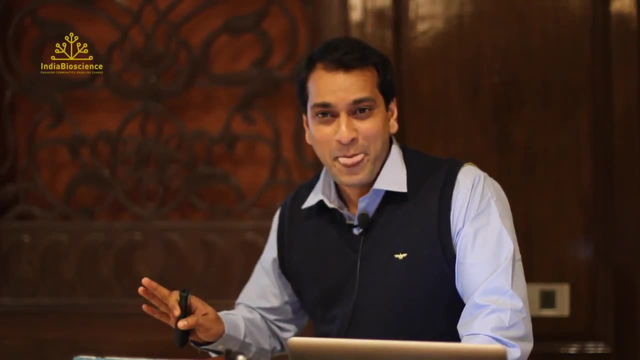 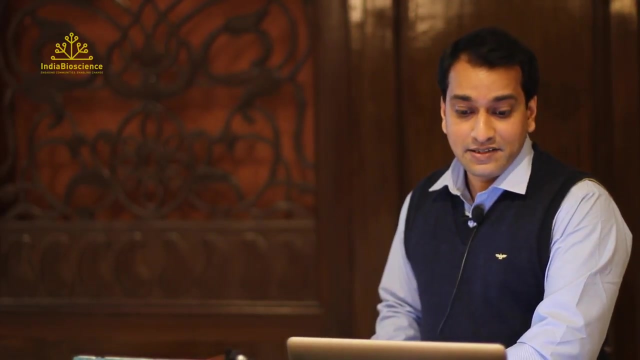 Some of them completed And a few of them are currently under review. I was afraid to show this slide today here because I know a lot of representatives from DVT DST are here and so are the reviewers, But nonetheless, writing grants and preparing grant challenges is very, very important early. 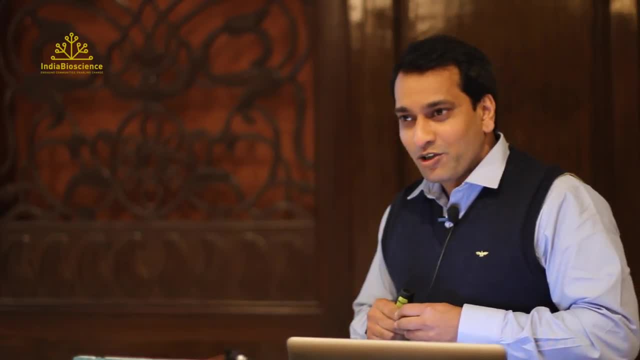 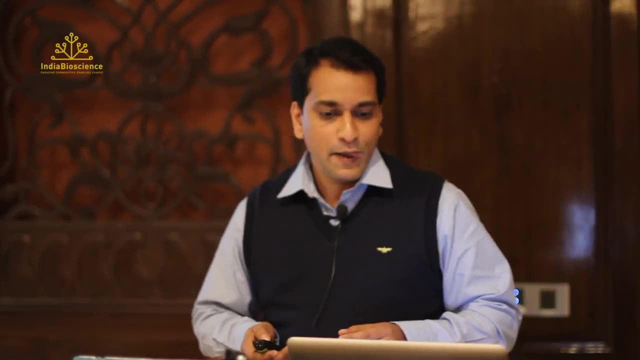 in your career. So what have we done with all this money? I am just going to give you two areas of work where we think we have made a very small difference. First, we have done a lot of work. The first approach is something called as capsid bioengineering with the AAV vectors. 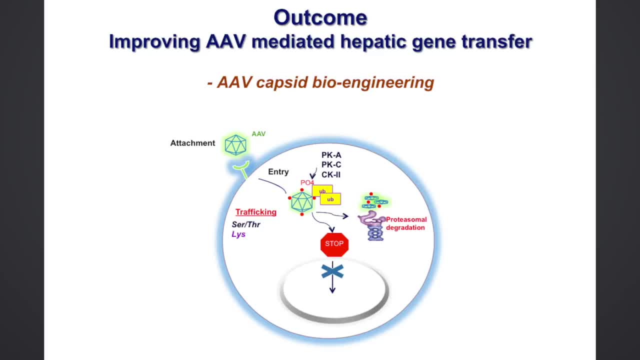 The hypothesis goes something like this: We reason that once the AAV vectors are internalized into the cell, the cellular cytoplasmic surveillance machinery through the serine-threonine kinase enzymes- the kinase enzymes selectively phosphorylate this viral capsid protein. 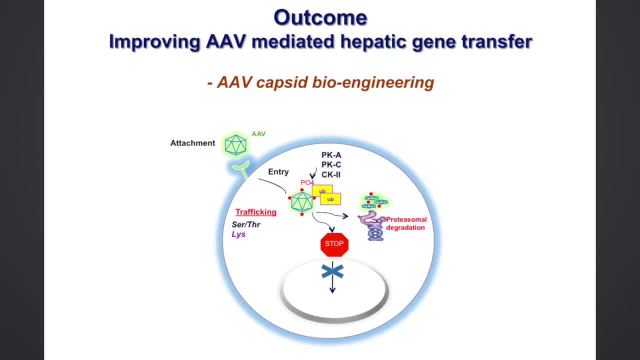 And this serine-threonine phosphorylation seems to act as a cue for ubiquitination of the viral capsid. And this ubiquitinated viral capsids are then proteosomally degraded just like any normal foreign proteins would be. What this meant was the net loss of the number of viral particles that could enter into the. 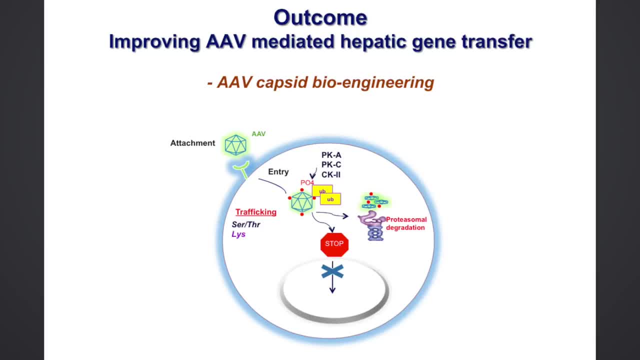 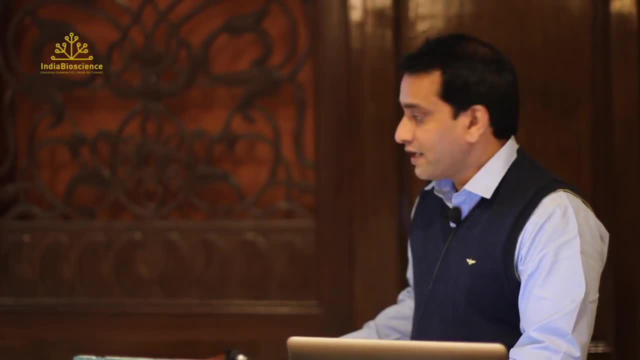 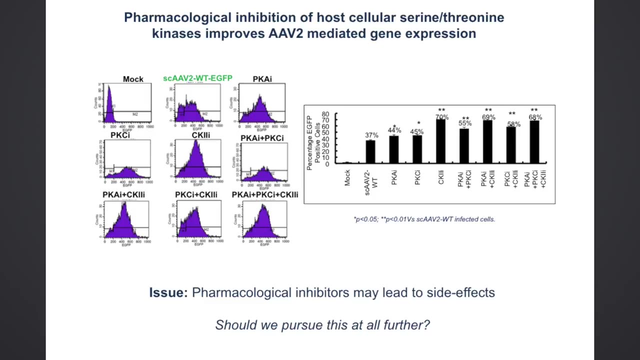 nucleus and affect its gene expression. So the simple way to check it: pre-treat the cells with inhibitors against this serine-threonine kinases and see what the output was. And this is precisely what we did When we did this. this is the gene expression from wild type vectors. 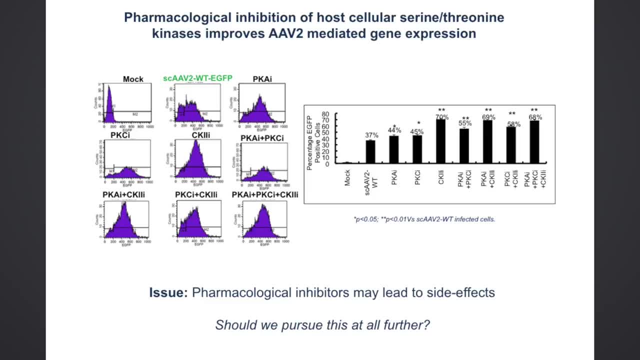 These are various serine-threonine kinase inhibitors that were used, And the gene expression roughly doubled Showed that, yes, indeed, they were playing some role here, But, as you all know, serine-threonine kinases have multiple cellular functions, so we were 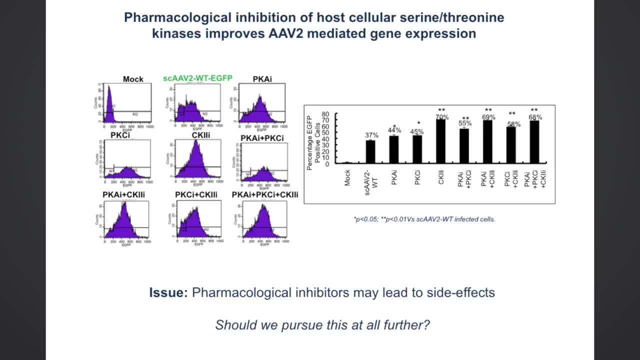 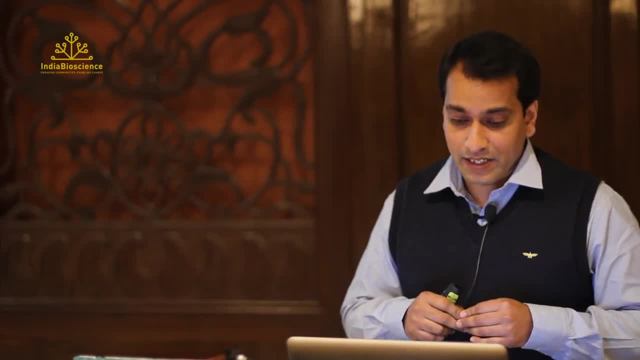 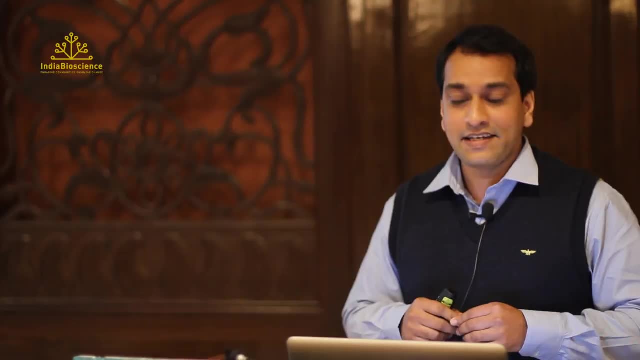 kind of worried about the side effects. So what we did was if you were to scale. so the question was: should we pursue at all with this further? This was the first major challenge we had, And I realized that when we are stuck in a research interval, talk to your peers and 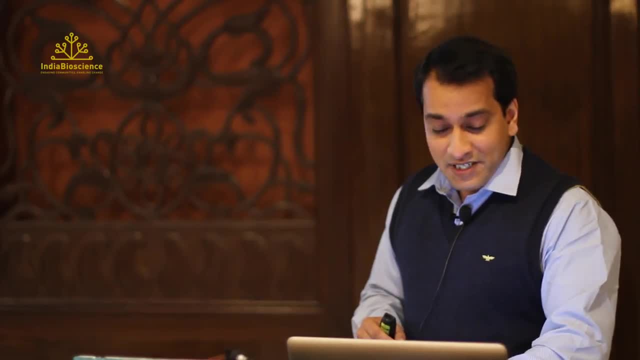 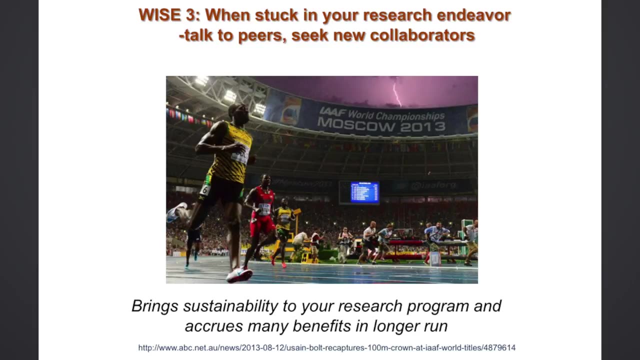 seek out new collaborators And I must thank. and it brings sustainability to your research program and accrues many benefits in the longer run. This was not the longer run, This was the 100 meters in the IAF at MASCO 2013 championship. 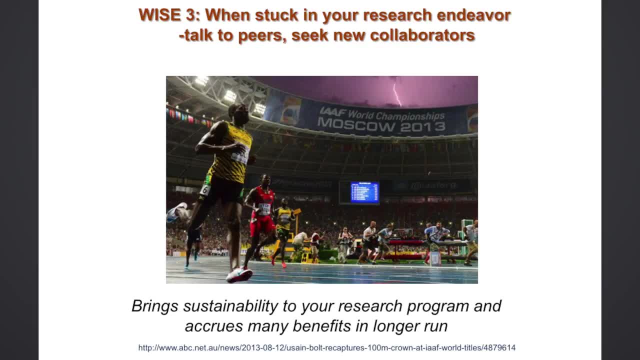 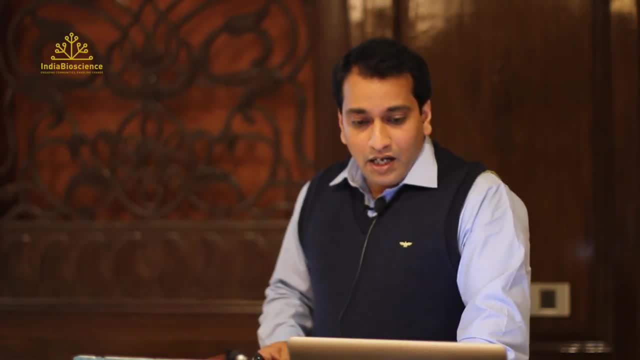 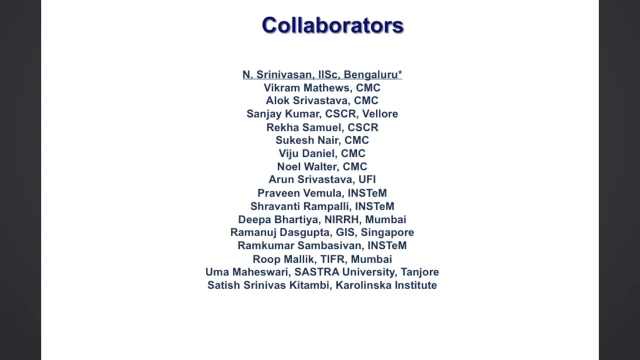 And you can see here that the lightning bolt was made by the natural lightning And it was a very famous picture at that time. I must thank all my collaborators, who are all listed here, And there are also very formative collaborations that are currently ongoing which are not listed. 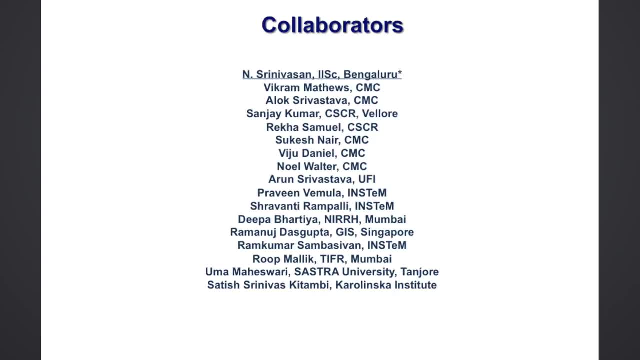 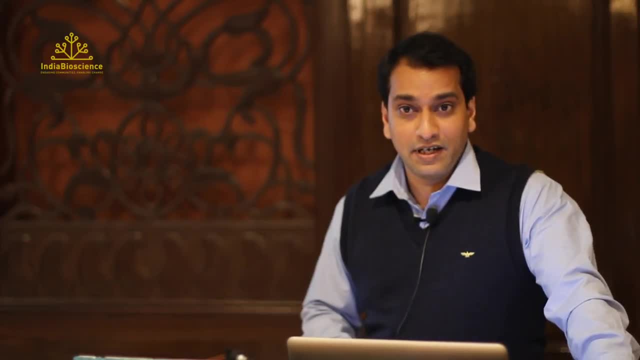 here I would like to make a special mention of Professor N Srinivasan from ISC Bangalore. I approached him early in 2010.. I didn't have my grant just three months into my new position And I said: I have a problem like this. 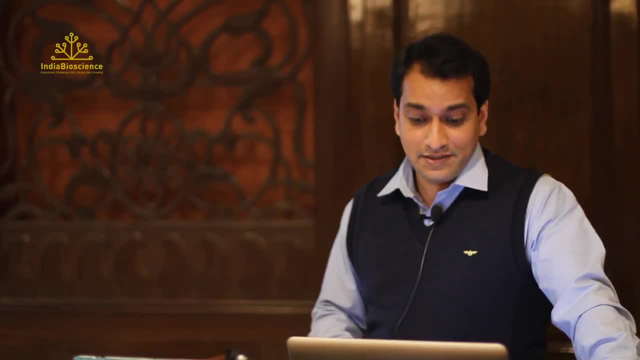 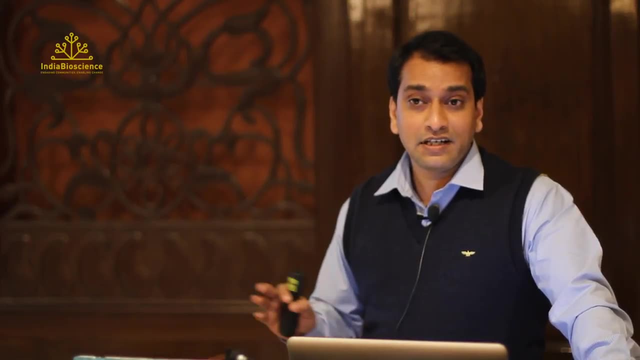 Your lab works on serine-threonine kinases. My lab was just being set up- no independent publications, no grants- And he said, within half an hour of sending the email stat came the reply: can we meet in ISC within the next two weeks? 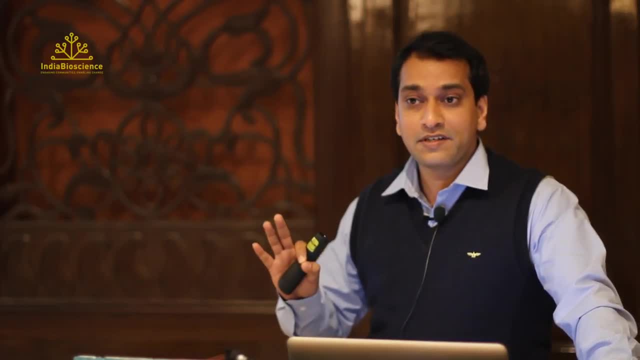 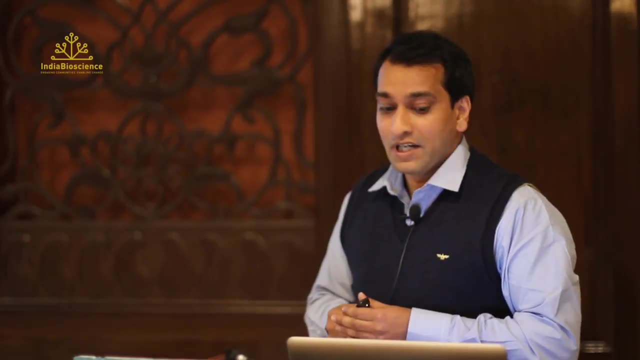 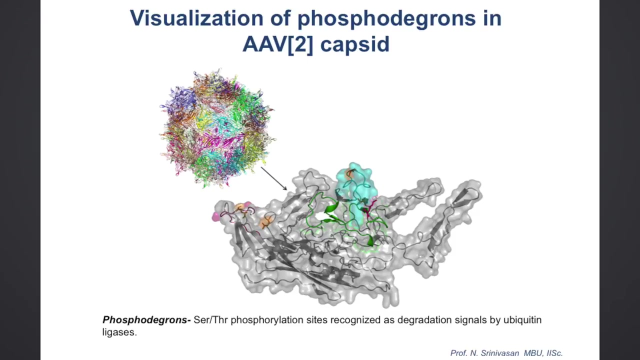 Off we went And now he has been a source of immense professional support for the last five and a half years. So these collaborations help you a long way. So they helped them identify what is called as the phosphodegrons, or a cluster of serine-threonine. 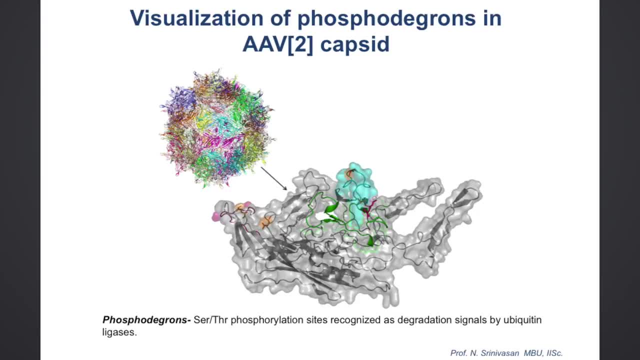 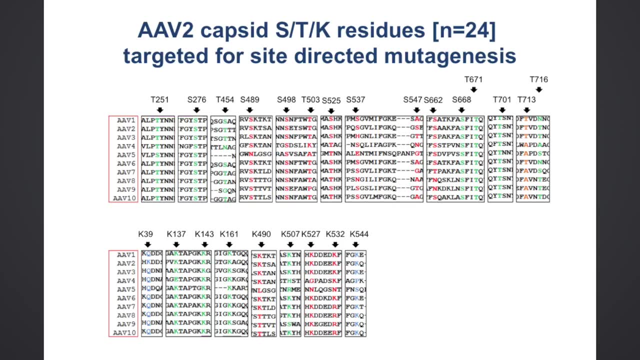 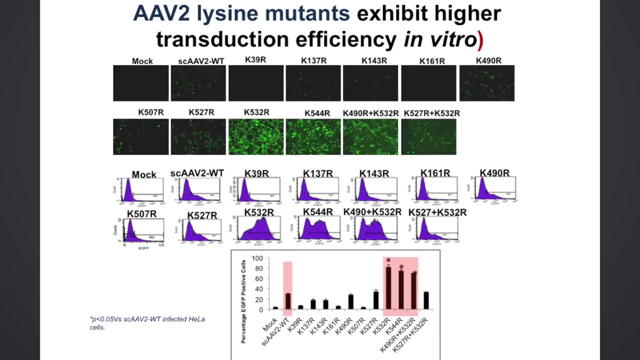 phosphorylation sites in the AAV viral capsid. Three such phosphodegrons were identified, And then we mutated residues- amino acids- In and around this phosphodegrons. What was the outcome of this? We were able to improve the transin expression from somewhere here to somewhere over here. 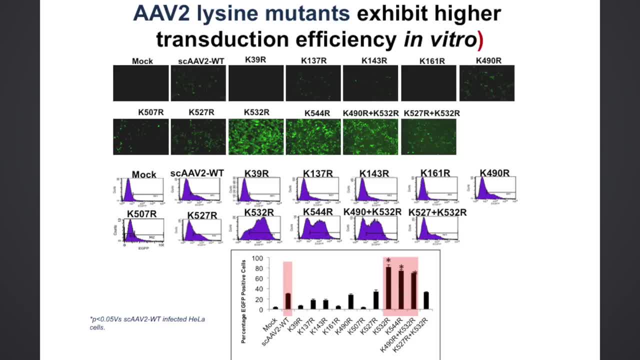 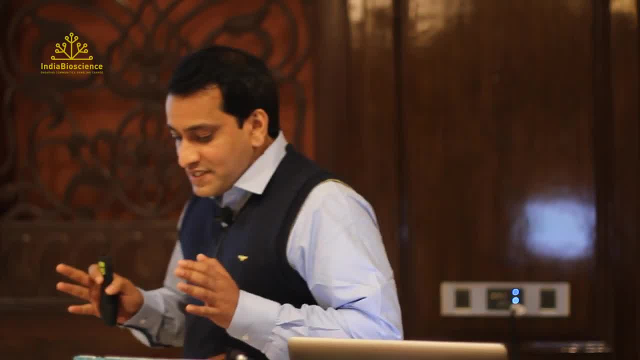 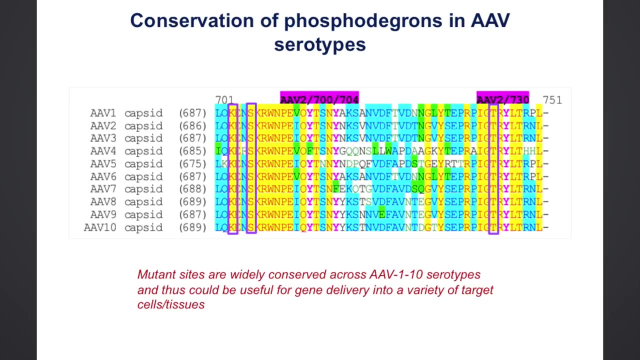 roughly about three-fold increase when you look at cells that were transduced. So this was in cell lines. The biggest advantage of this approach that we took was that the residues that we started modifying on the prototype virus, which is AAV2, was conserved in all the 10-0 types. 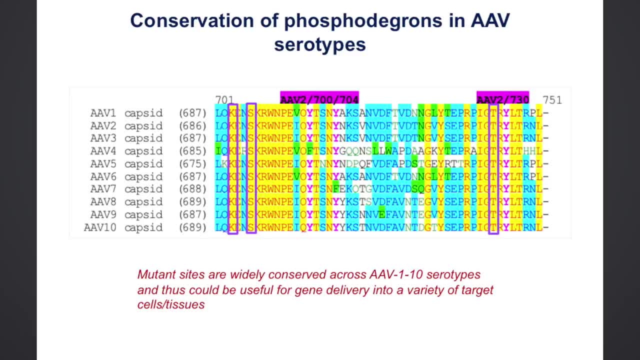 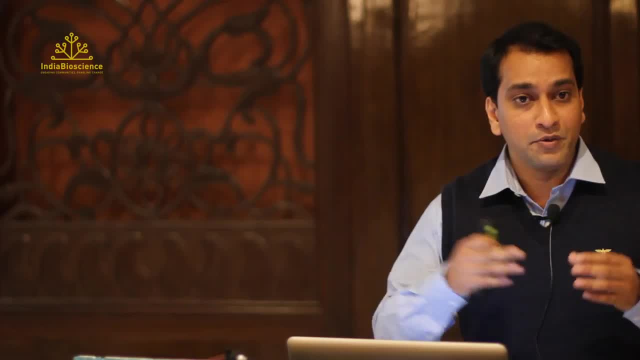 Which meant now you could not only create liver-specific viral vectors which are better in terms of performance, but also vectors which are good for cardiomyocytes targeting or for lungs, so on and so forth. I'm just going to show you some brief examples. 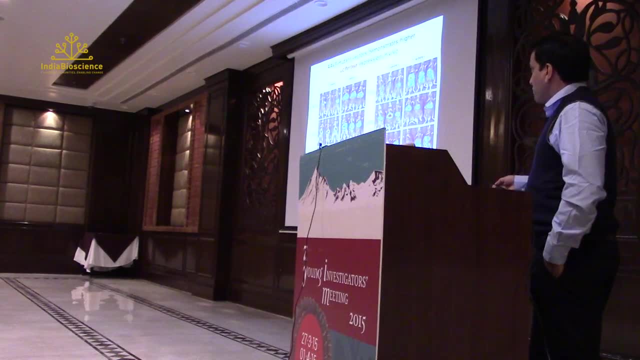 This is with reference to AAV8.. This is the hepatic gene expression. you see with the unmodified vectors And this is what you see with some of the modified vectors: A modest increase, but still a significant increase of about two-thirds. 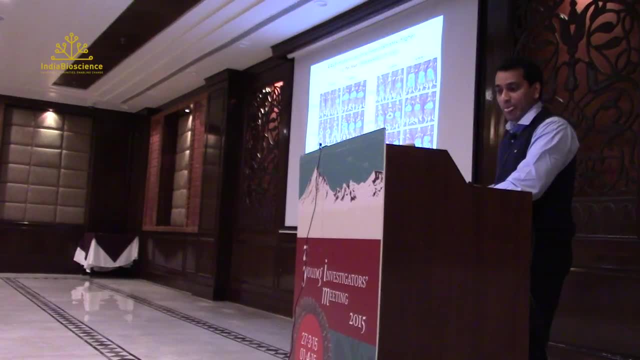 Of about two to five-fold, with different members in the lab, And then what we did was to collaborate with the groups that performed the clinical trials. We got the clinical trial vectors whose Factor IX expression was somewhere over here And we tested the transgenic hemophilia being matched. 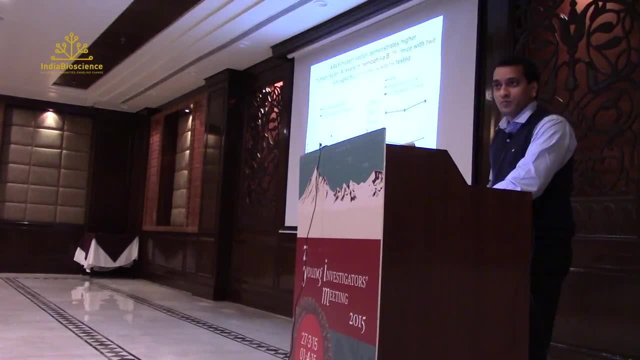 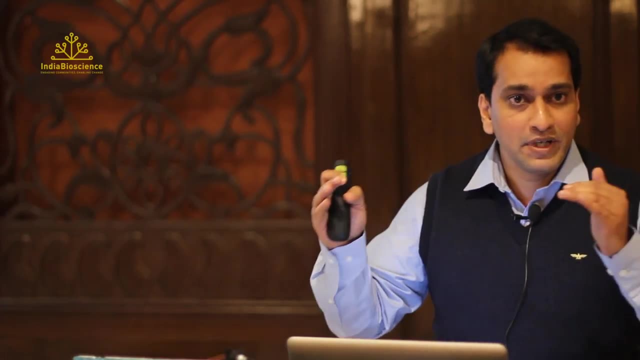 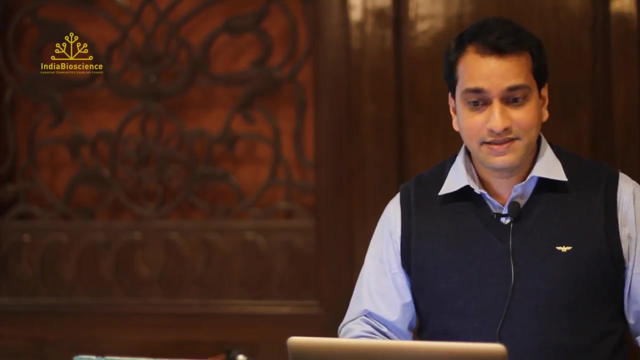 And what you see with our vector systems is much improved performance. So this is in terms of whatever we did In terms of improving the efficiency of the viral vector system. The second approach was how to tackle the pre-existing immunity that is seen in humans. 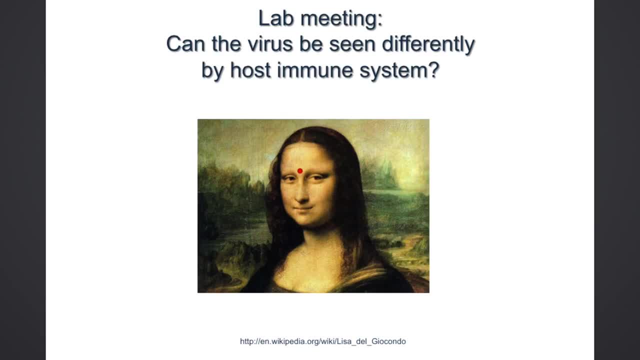 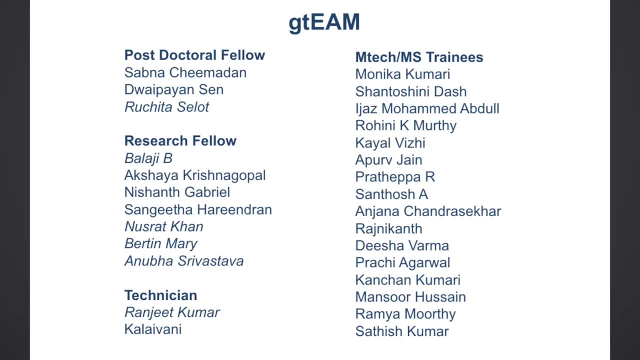 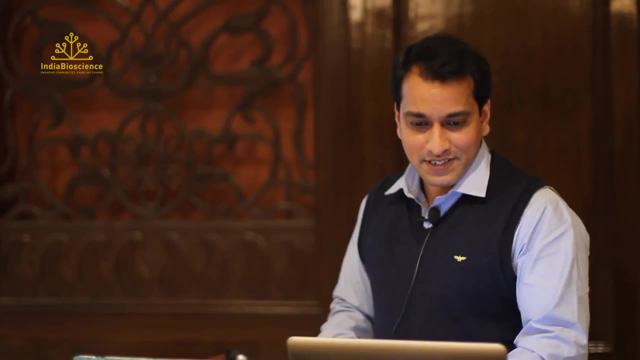 So we have these lab meetings every Monday. So I asked the people: can the virus be seen differently by the post-immune system? Something like this: So this is my group, pretty smart group, You can't beat them. And so then the follow-up question was: can we mix and match some of the AAV8 we want to use? 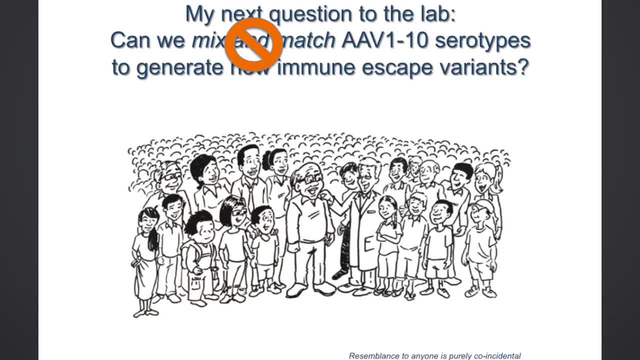 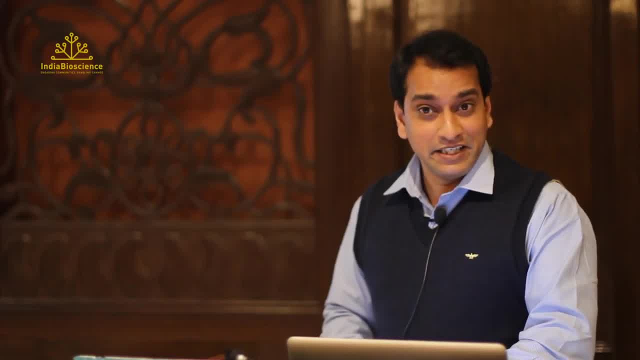 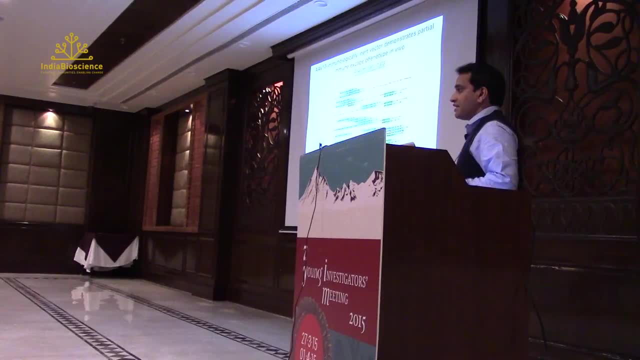 Can we do 10 serotypes so that we can achieve this immune evasion which is specific to each serotype? So they rejected my idea. They said no way. But they gave a good idea in a sense. They said: why can't we map all the antigenic epitopes? 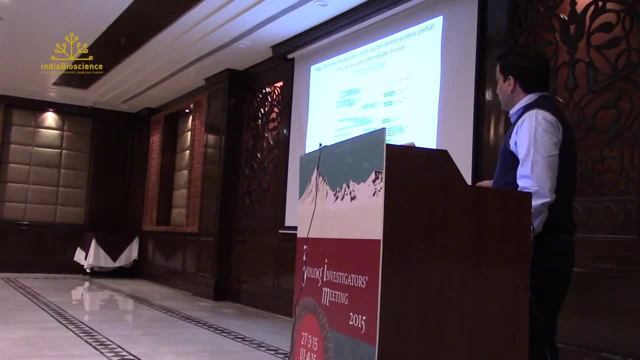 Potential T-cell and B-cell antigenic epitopes in the AAV capsule. Try to knock them off one by one and see what happens to the data. And this is what we achieved. This is very promising information, but very preliminary information in our efforts towards making this vector a universal gene therapy vector. 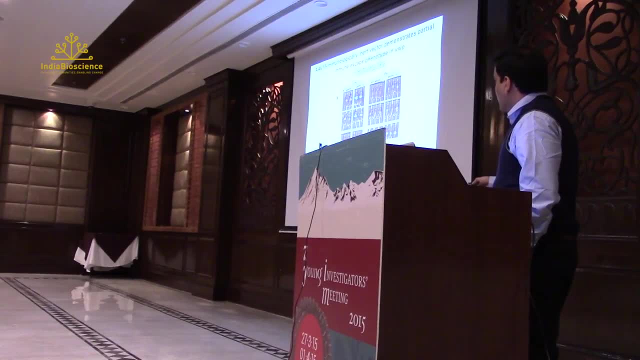 As you can see here, these are representative animals And these are animals treated with the wild type AAV10 serotype vectors, When you pre-treat them with intravenous immunoglobulin, which is nothing but donor pooled serum that contains anti-AV antibodies. 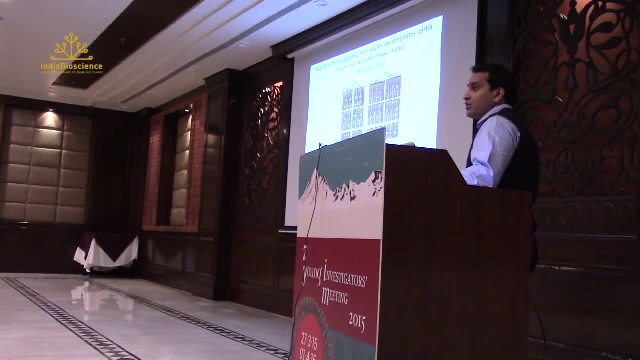 the gene expression is completely lost. But, however, when we use these mutant vectors, which are immune escape vectors, the gene expression is partially restored. So this was very promising. We are now doing elaborate studies to identify what are the other mutations that we could add. 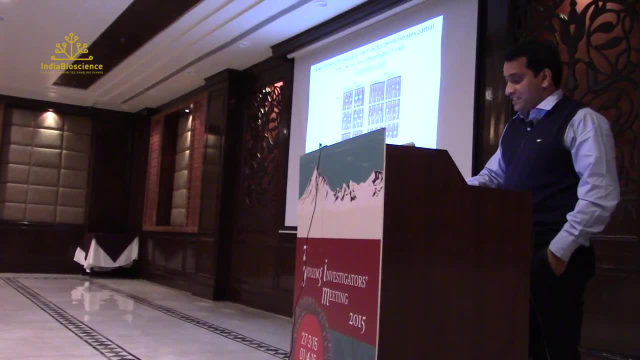 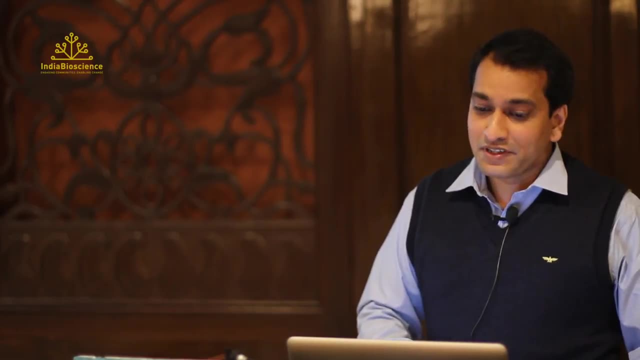 so that this becomes a universal gene transfer vector. 5 plus 4 is 9, and so is 6 plus 3.. One of the things that we have, I have realized, Many of us have realized this: Appreciate your people's ideas. 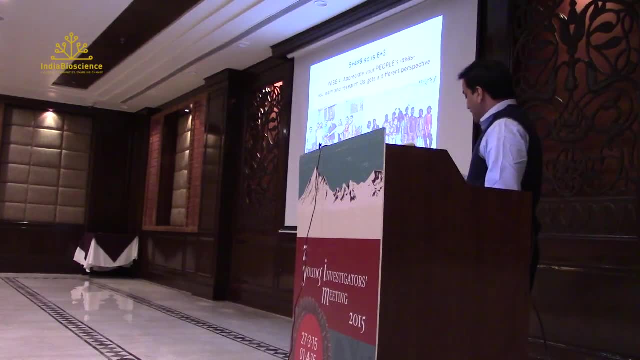 You learn and get a different perspective. Same set of students before and after their holy celebrations Got the same numbers. So we generated AAV vectors with modified phosphodephrons and we are also trying to make this system universally applicable. I am going to slightly shift gears and talk about 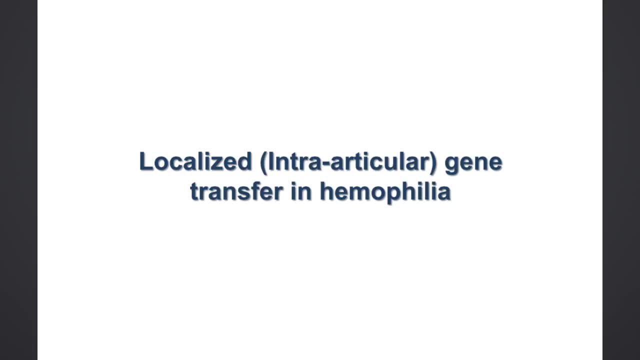 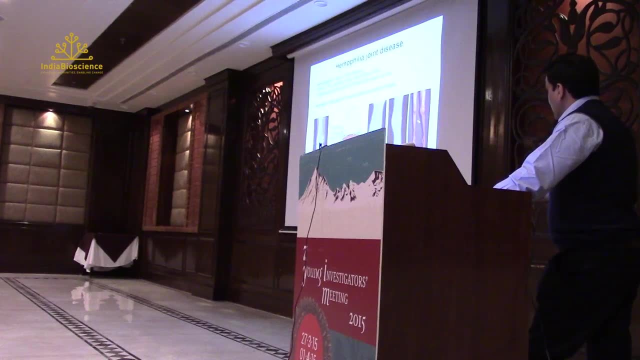 our other contribution to this field of research, which is intra-articular gene transfer in hemophilia. Now, the development of arthropathy, which is something like this, is a major comorbidity in patients with hemophilia. Why does this happen? 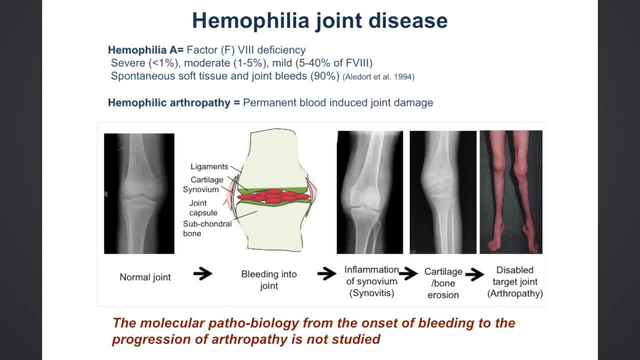 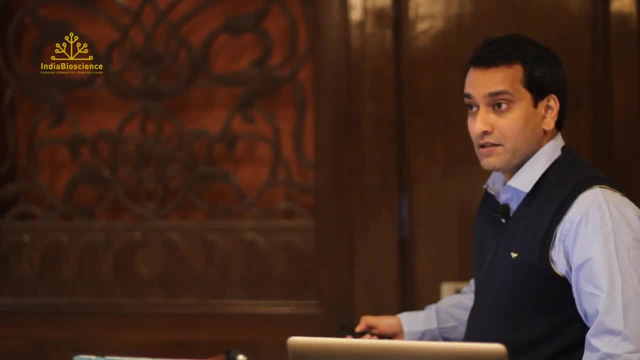 You have repeated bleeding episodes in the joint. In a normal human being, if you have a traumatic bleeding, the excess blood is reabsorbed by the synovial lining here. But in case of hemophilias they spontaneously and recurrently bleed into the joint cavity. So once you have four to five bleeding episodes, the synovial loses the capacity to reabsorb blood from the joint cavity. It becomes inflamed to result in synovitis. Over a period of time it affects the articular cartilage. 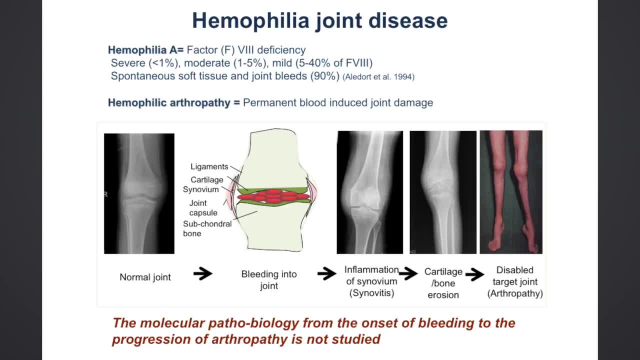 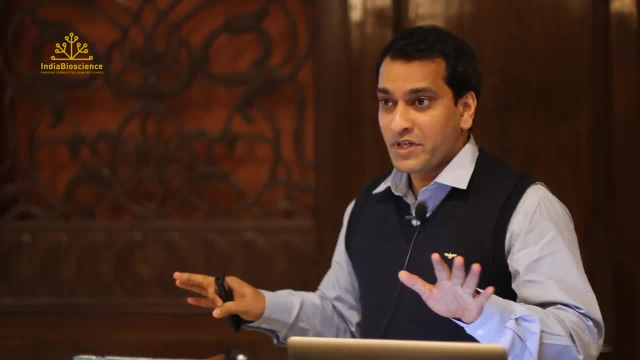 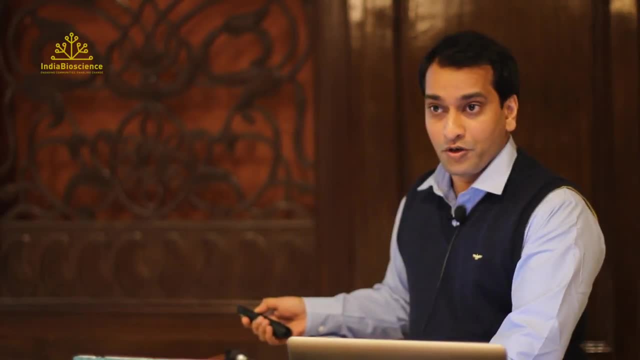 to lead to a condition called a target joint. This is basically your femur and tibia. without the articular cartilage It is like driving your automobile with deflated tires- Pretty painful. So the molecular pathology from the onset of this process to here is not known. 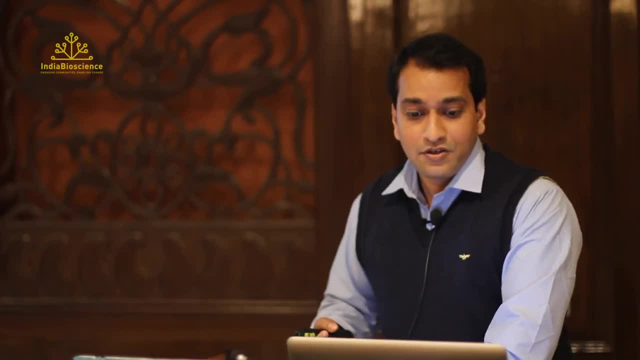 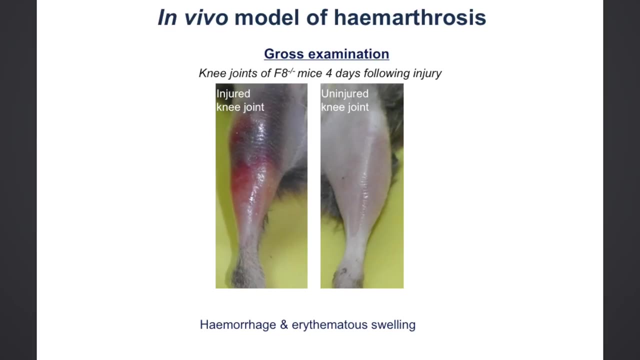 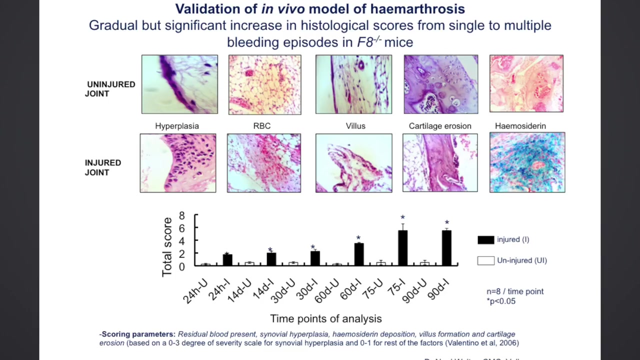 because of ethical considerations in obtaining these tissues. So what we did was we improvised. We took transgenic mice, We recreated the conditions that we see in humans by joint needle injury. We validated them basically by histological analysis: All characteristics, what you would see in a target joint. 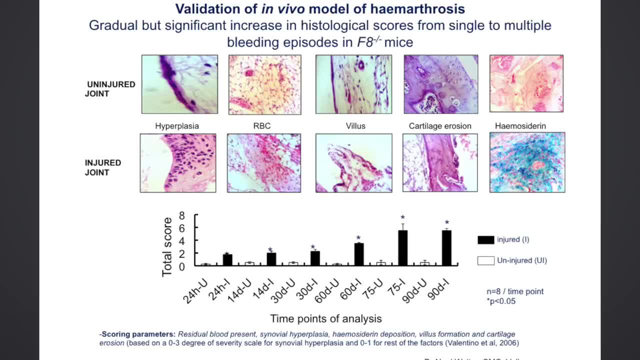 like synovial cell hyperplasia. the RBC deposition, Willis formation, cartilage erosion and hemocytin deposition is seen here And progressively the joint's force worsened in the injured joints for a follow-up time of three months. 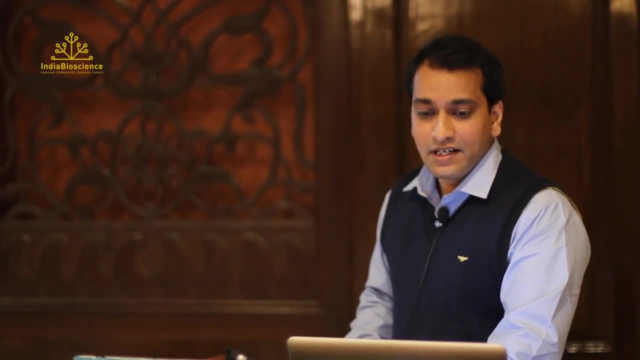 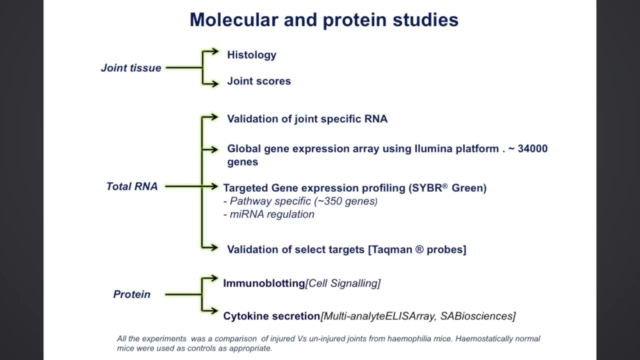 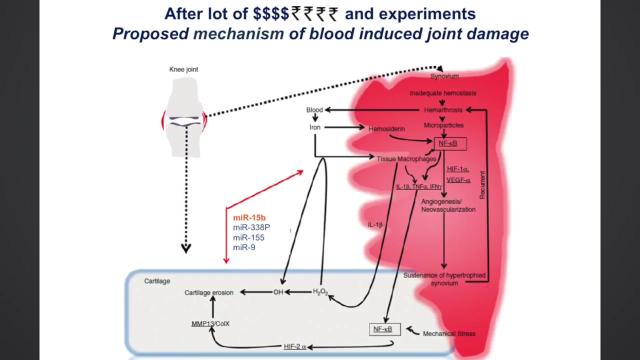 Now with this validated set of animals. we lost quite a bit of money as well here, but we did quite a bit of work And then finally came up with this speculative model, partly supported by our data, which is when there is repeated bleeding episodes into the joints. 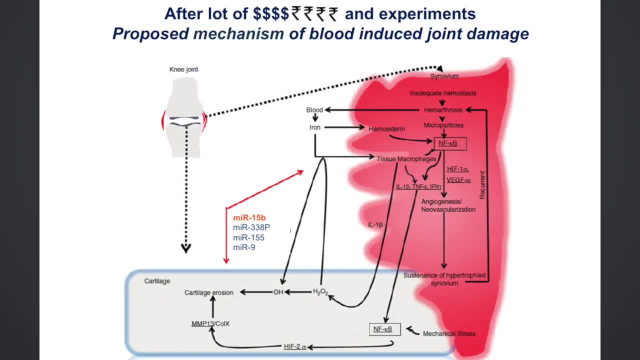 the RBC gets deposited here And the breakdown product of RBC is hemocytin. Hemocytin seems to activate pro-inflammatory NF-kappa-B. NF-kappa-B has multiple. it's a transcription factor, as you all know. 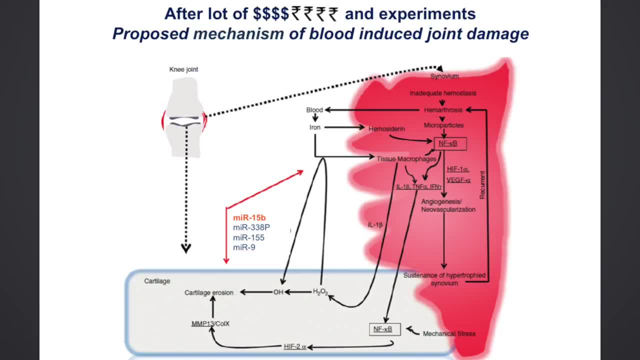 has multiple targets, activates pro-inflammatory pathways, pro-antigenic pathways and also pro-hypoxic pathways. This leads to the formation of new capillaries and which are friable and break easily with minimal stress, as it happens in the joint. 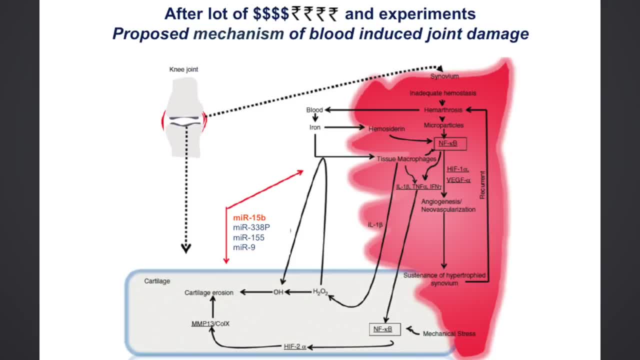 So this leads to recurrent phenomena of bleeding, NF-kappa-B activation, pro-inflammation and angiogenesis in the synovial Over a period of time. this affects fills on to the articular cartilage, affects the expression of. 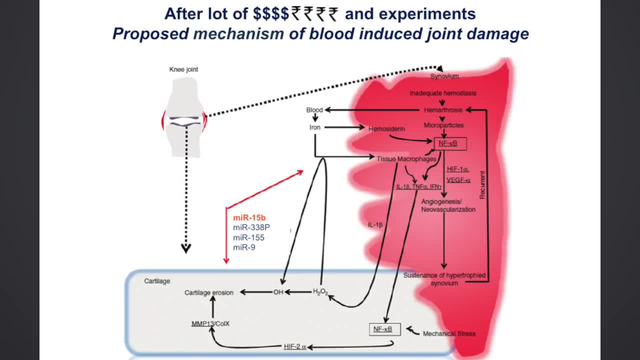 increases the expression of matrix metalloproteinases, which are articular cartilage degrading enzymes, And several microorganisms were found to play a role in this process. One of these microorganisms was very interesting, 15B, because it is known to act against both. 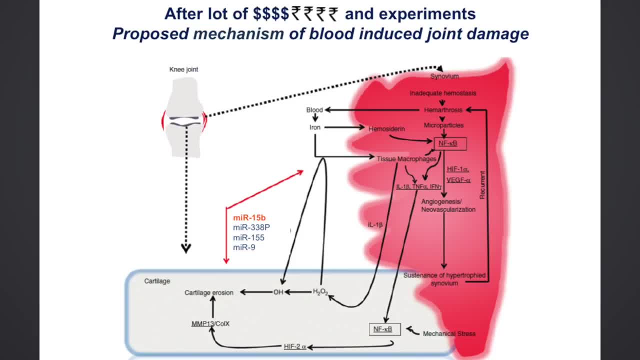 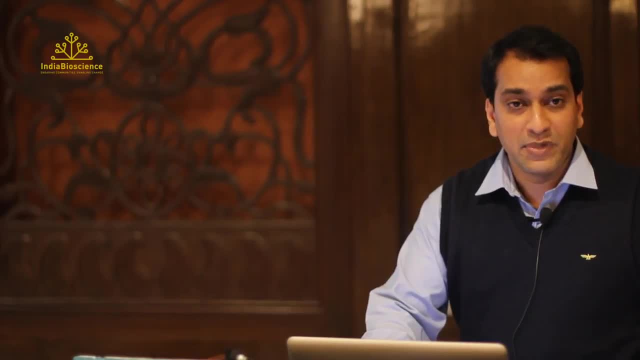 wedge of alpha, the pro-angiogenic factor and also the hypoxic inducing factors. So we asked the question: can we reconstitute the levels of this particular protein in the joint by intra-articular gene transfer method and see what happens to the phenotype? 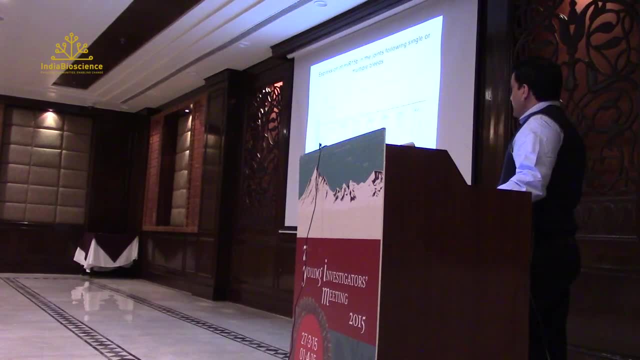 So a closer look at the microarrhythmia 15B expression levels would show, after each bleeding episode, which the levels of this particular microarrhythmia was going down in animals which were bleeding. So we then developed AAV vectors which were used to specifically target. 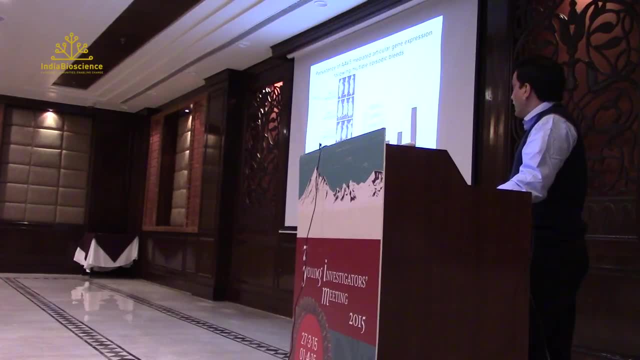 the microarrhythmia 15B into the joint cavity And once we did this, we could see a considerable reduction in terms of pro-angiogenic factors and hypoxic inducing factors And the joint inflammation scores significantly reduced in this animal models. 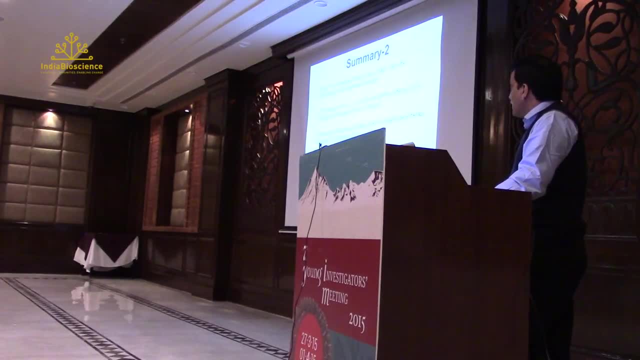 treated with microarrhythmia 15B as well. So NF-kappaB and its associated factors we had shown play a major role, and intra-articular gene transfer of one of the microarrhythmia seemed to at least improve the phenotype. 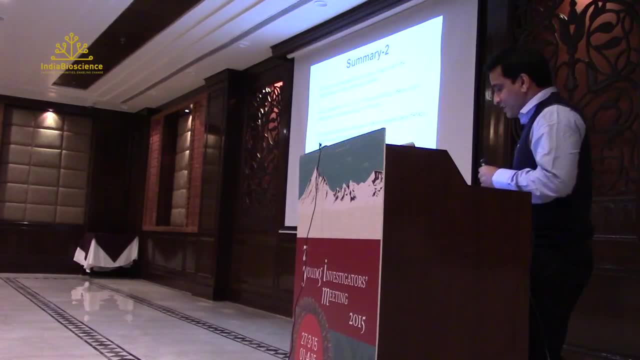 of hemophilia arthropathy. However, further elaborate studies are going on because I firmly believe no one microarrhythmia can regulate a single pathway. so we are also trying to map out the other microarrhythmia which could play a role so that we can develop. 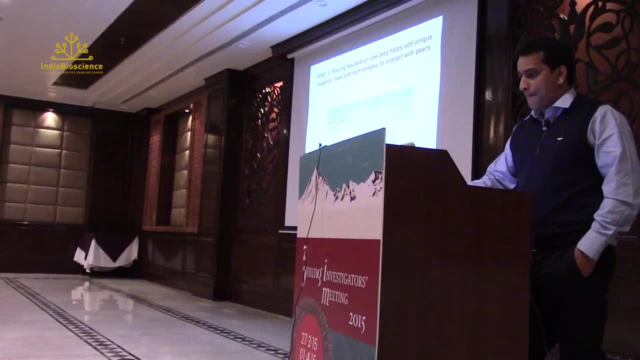 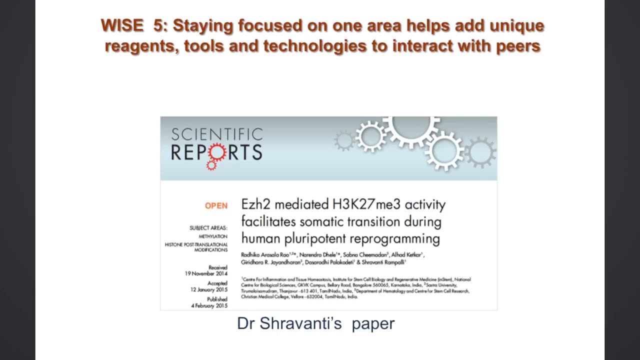 a combination gene therapy protocol. This is Dr Shravanthi Sreepur, and because we were developing AAV-based microarrhythmia systems, we could help her project, which otherwise we would have never gotten involved, in pluripotent reprogramming. 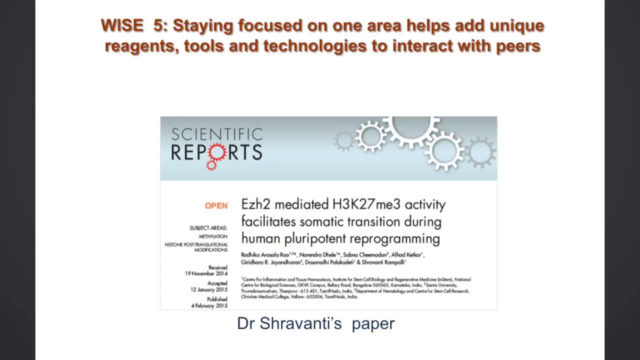 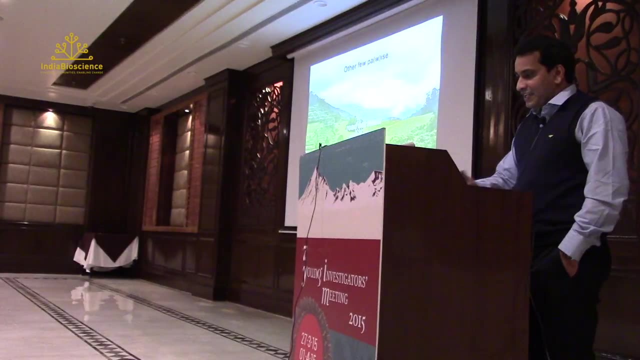 And we could actually give some of the microarrhythmia constructs that we developed to test in her own systems. And basically the message is: staying focused on one area helps add unique reagents, tools and technologies to interact with your peers. This is my other two cents. 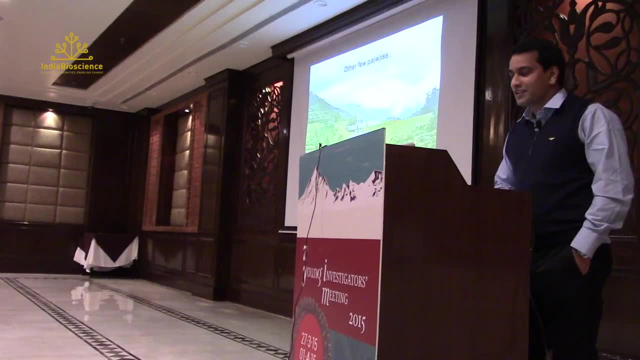 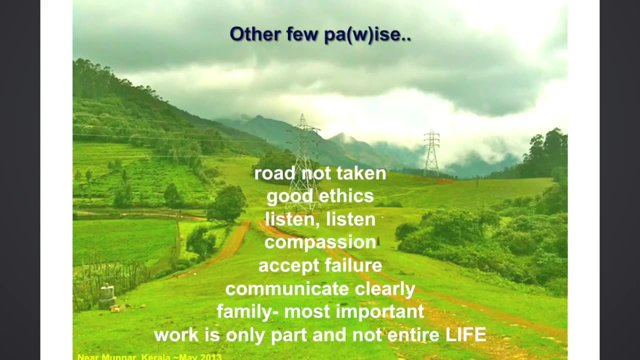 Whenever I write a project, I try to take the route that was not taken as much as possible, So you have higher chances of success with your projects. Of course, good ethics of what you do and what you preach and what you practice is very, very important. 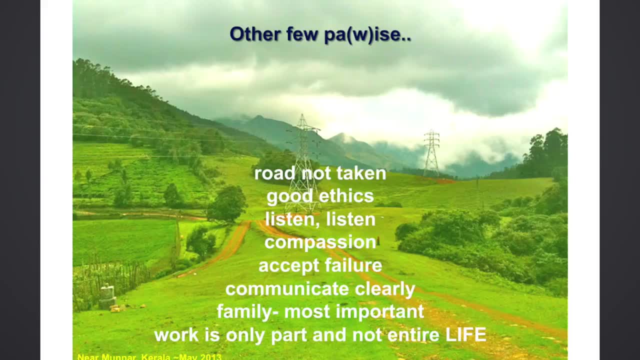 Listen to your colleagues, Listen to your students, more importantly, And please approach them with compassion. Not all five fingers are the same. You could have multiple issues. Management is the biggest issue when you want to become a mentor or when you are already a mentor. 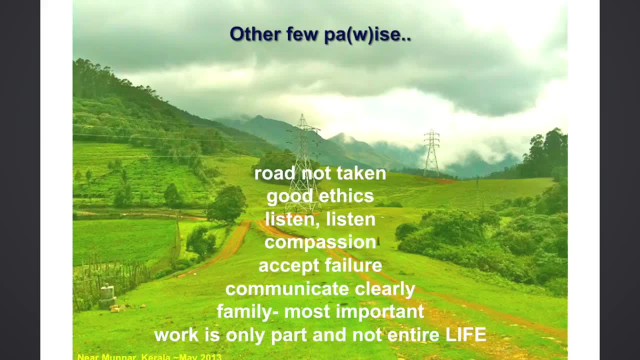 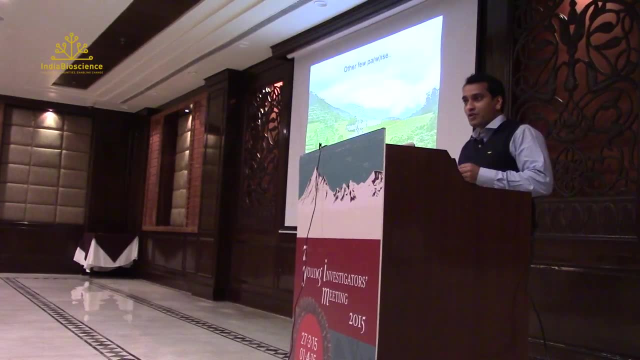 I still haven't figured out how to do it And I fail all the time. So accept failures, Communicate clearly. This is very, very important. I think Not only to your peers, supervisors or your own head of the departments. 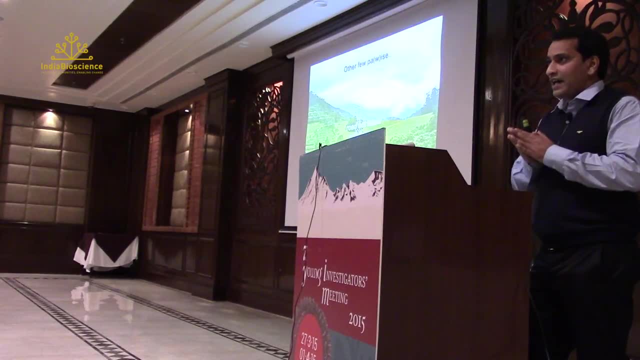 also to your students. Tell them very clearly: I need one, two, three. Do you have any issues in doing this? And if there are any issues as a mentor, it's your job to clarify it, But otherwise, communication is the most. 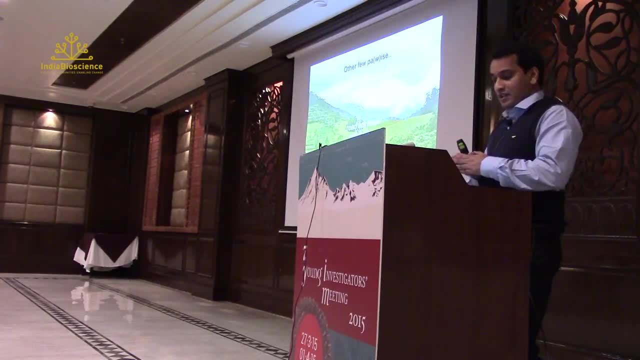 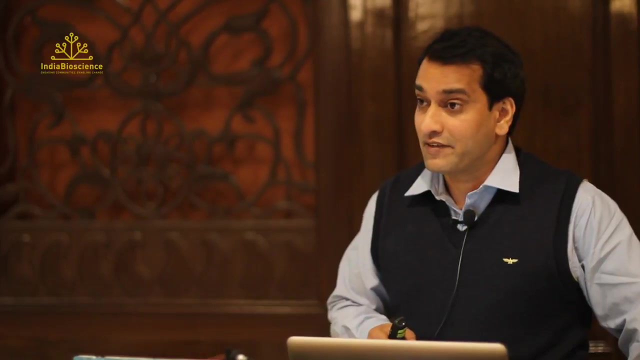 most crucial component of doing good research, And family is the most important component. It's an understated component, but unless you're the PI who, by yourself, are happy, I think we have to see things as work is only part of life and not entire life. 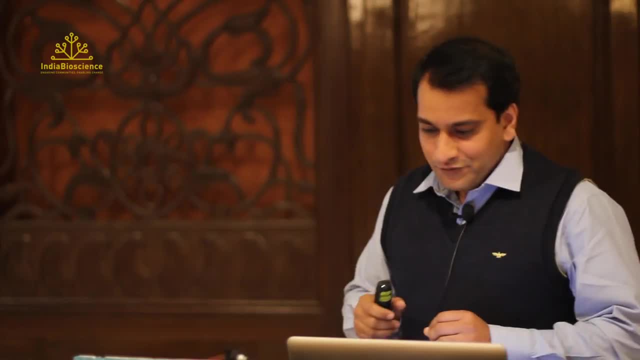 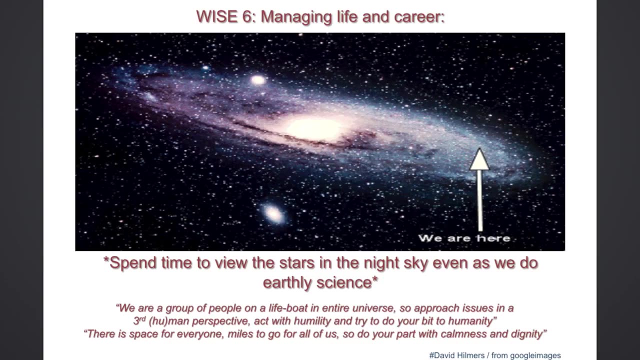 To illustrate this. we are somewhere here, a speck in this big galaxy with hundreds and thousands of galaxies, As we are trying to do, remarkably, earthly science also spend time to view the stars in the night sky And, to quote what I heard a couple of weeks ago, 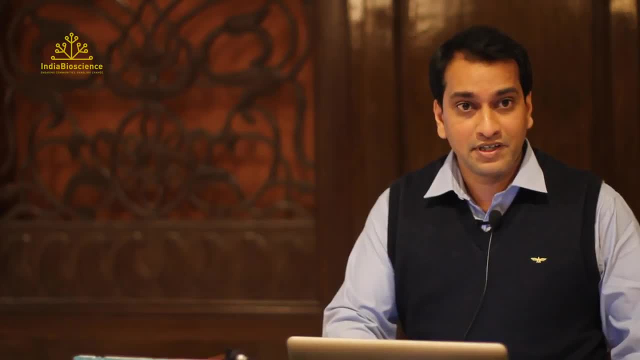 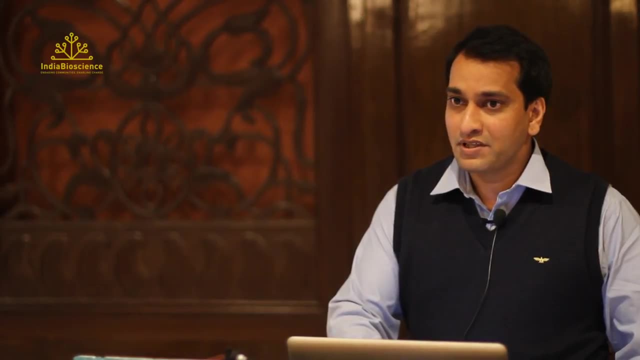 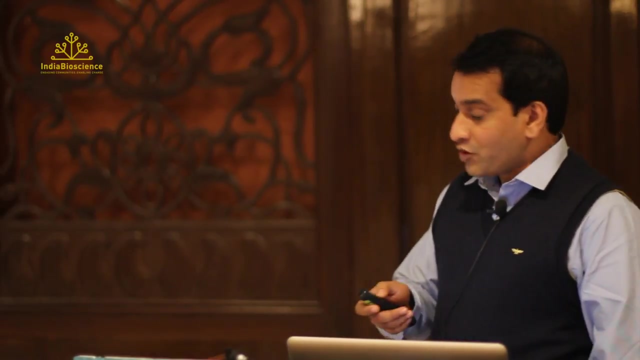 from Dr David Hilmes, who was a former NASA astronaut. now he has done his medicine and he is doing charitable medical work throughout the world, including in Liberia, where you had an Ebola outbreak. And this is what he said and I'm quoting him: 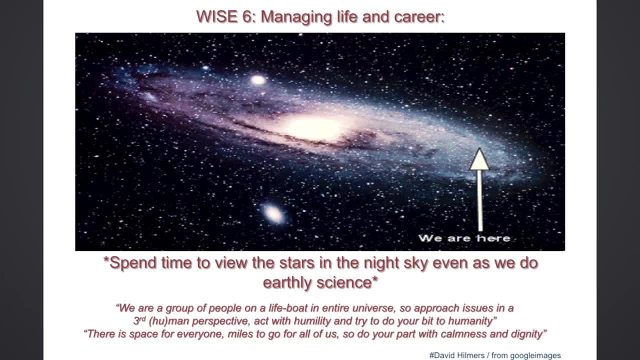 we are a group of people on a lifeboat in an entire universe. So approach issues in a third human perspective. act with humility and try to do your own bit to humanity. And there is space for everyone. miles to go for all of us. 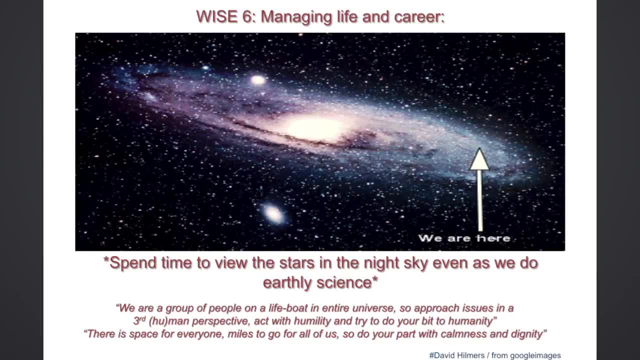 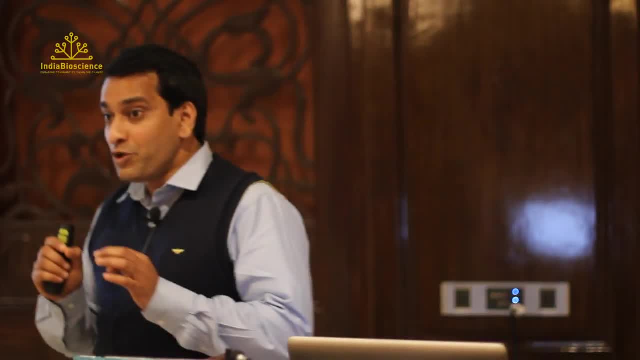 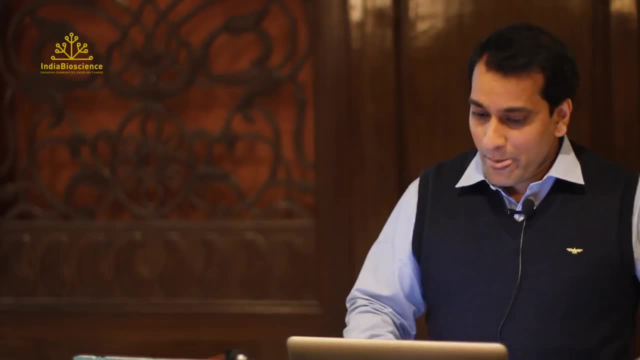 so do your part with calmness and dignity. This is so apt for anybody. However, if there is one thing that you need to be aggressive, that is: don't be bogged down by naysayers. dream big. So we all know this man. 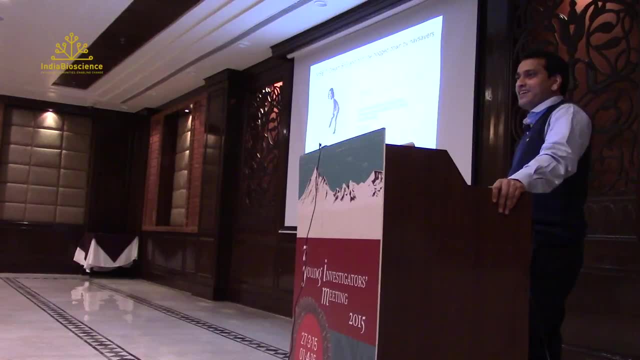 Sachin Tendulkar. He is a legendary figure and he had his own dreams, And very recently I found some interesting correlations between him and gene therapy. I wanted to share that with you. So Sachin Tendulkar was born. 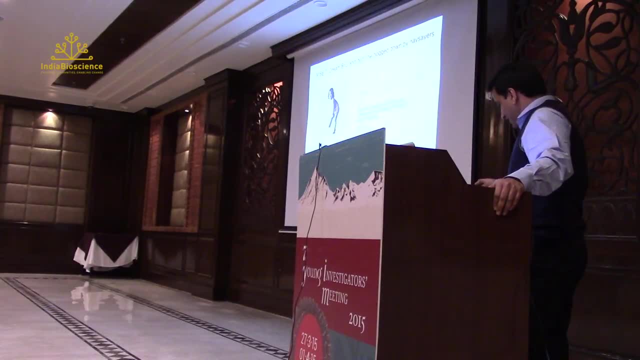 this was in 1973,, I think April. Gene therapy was still a myth When he made his debut, which is in 1989 in Pakistan, and Sachin Tendulkar and Michael Bliss and his colleagues at NIH were working out the protocols for gene therapy. 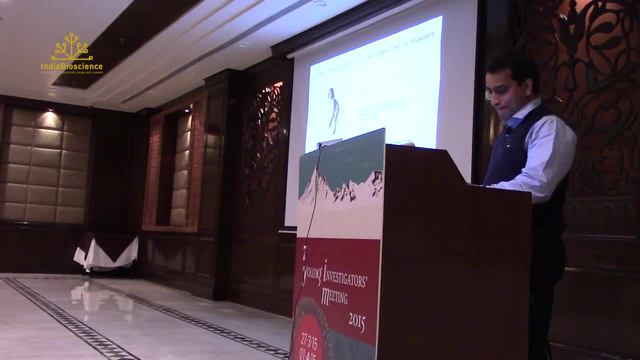 for severe combined immunodeficiency. So 1999 was a very bad year for Sachin Tendulkar. How many of you know cricket? I hope I am not going on a completely different tangent. So 1999 was a very bad year. 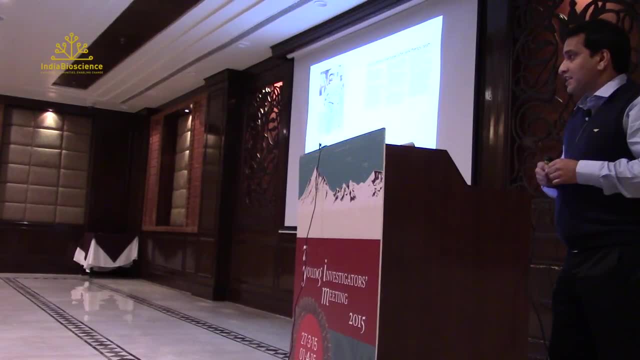 as far as Sachin was concerned, because his father died in the midst of the World Cup in England, He had to rush back, came back and then scored, essentially against Kenya. And that was the year you had a major issue in gene therapy, where all the clinical gene therapy trials 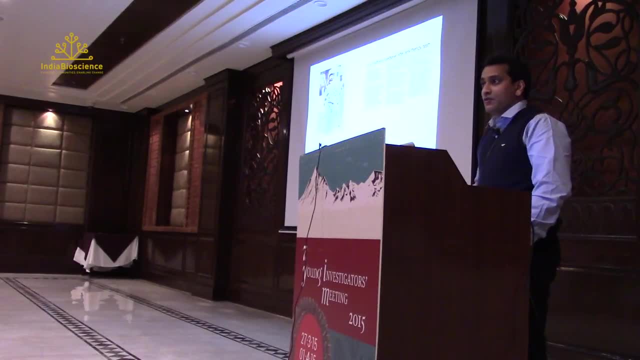 were put on hold because of the death of one patient, Jesse Gilsinger, who was treated for a condition called Mornithine Transcarbamylase Deficiency 2011,. India won the World Cup and the first successful clinical trial. 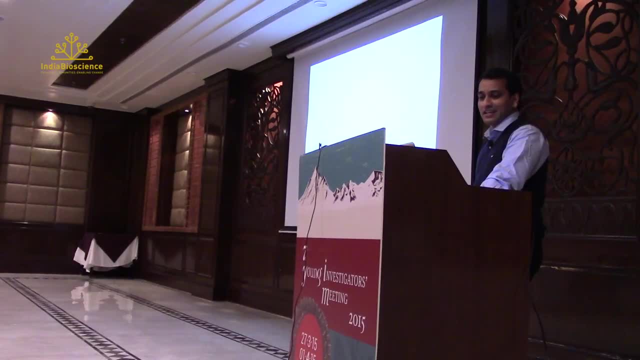 for Hemophilia B was published, And now 2013,, retired, good hairdo. the first commercial gene therapy product called Glybera has been licensed for a condition called Lycoprotein Lipase Deficiency within the EU. I know we lost in the semifinals of this World Cup. 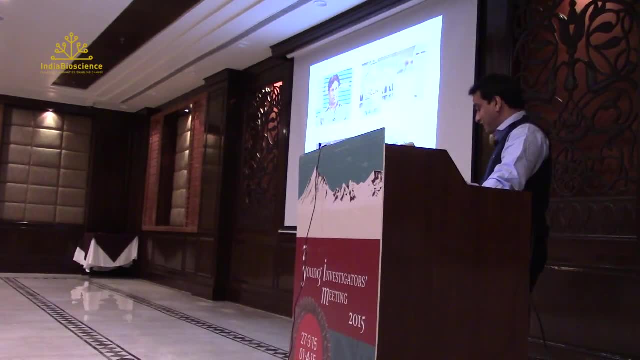 It's okay, But 2019, because he has seen failures. he has this habit of getting back in five minutes to the pavilion, But he has learned his lesson. I think he is dreaming big now to make it to 2019 finals.